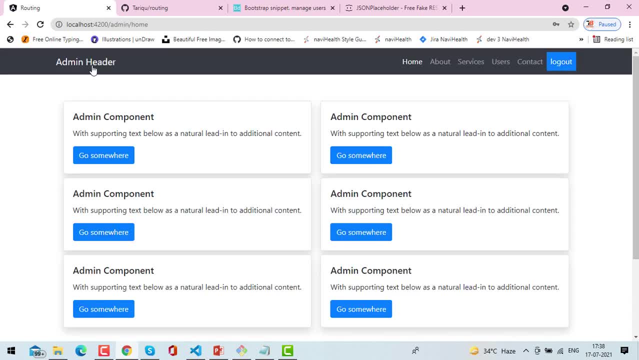 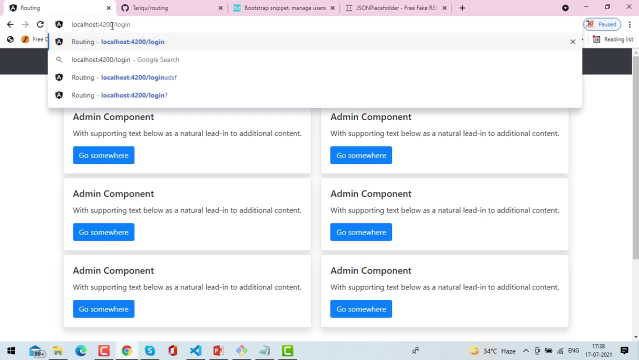 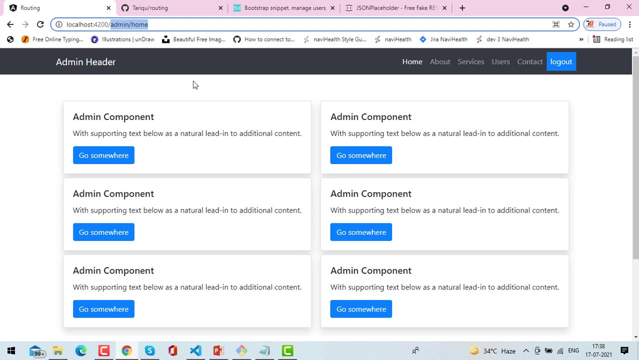 login Now. once user logged in, we'll take them to the admin page. Now. if user will try to go to back to the login page after authentication, then we will take them back to the admin. So it means once user is not logged in he can't come to this page. Once he's logged in, then he can't go back to the login. 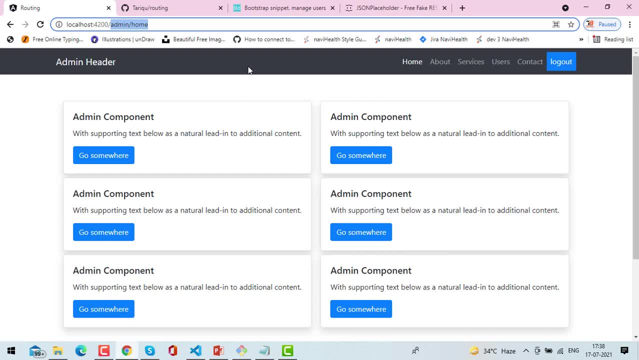 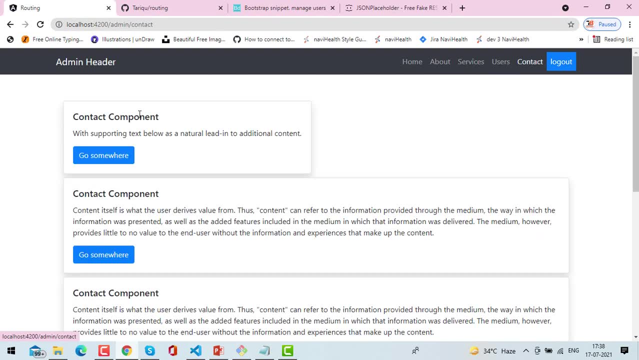 page. Okay, Now here you will find two things very common, like header and footer in all the routes. right, If I'll go anywhere, like about services, users contact, anywhere route is changing but header and footer are same, So we'll learn about multiple. 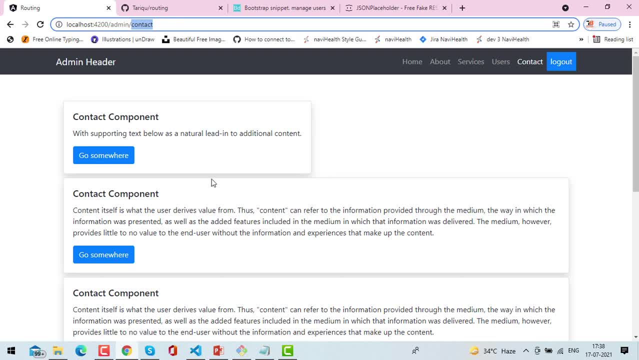 router outlet and we'll see how we could do child routing. So only the component is rendering here. header and footer are same. So let me clear one thing, guys: this video is not about designing. I'm not going to spend much of time on it If you want the same source code which I'm using in this. 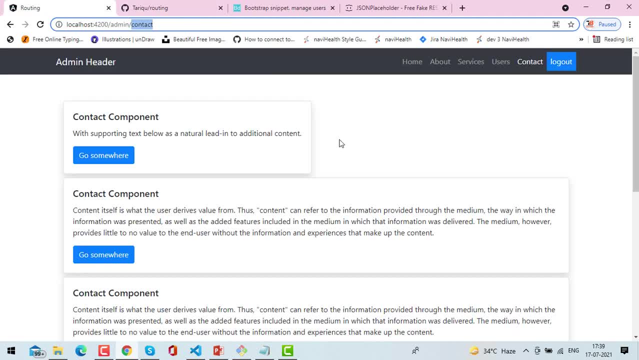 video. you can clone this project from my GitHub repository. So these are the things we are going to cover in this video And in future video we'll cover, like users, how we'll click on. then user will go to the admin page. So let's get started. So, let's get started. So let's get started. 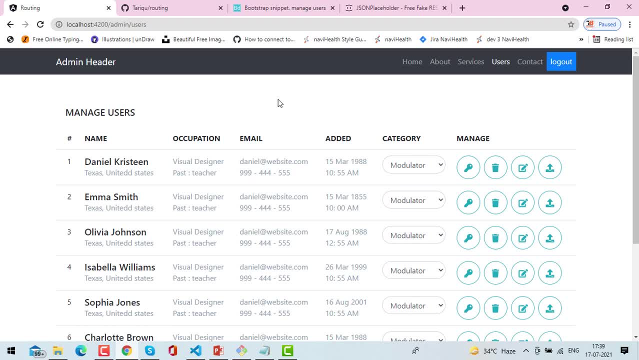 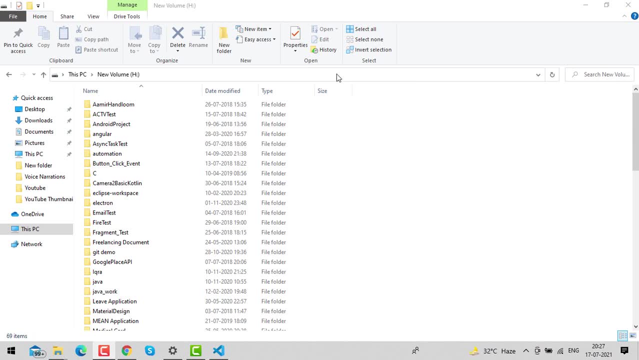 We'll go to the user detail page, like params and query params. We'll learn in future videos, So let's get started without any further delay. For this video, I'm going to create a brand new Angular project, So go to the folder structure where you want to create a project and type. 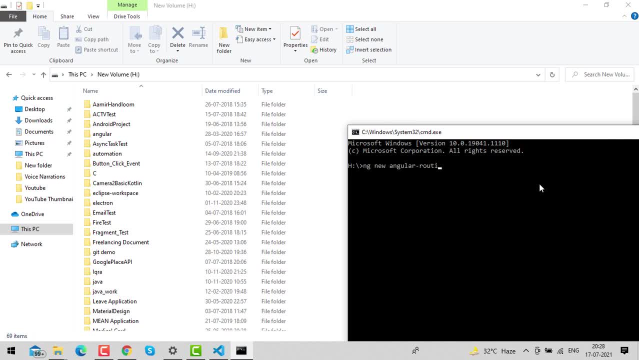 command engine: new Angular routing. It will ask few questions like: would you like to add Angular routing? Yes, this video is all about Angular routing- And then choose CSS, SCSS- I normally prefer to use SCSS file And then it will create all the files. 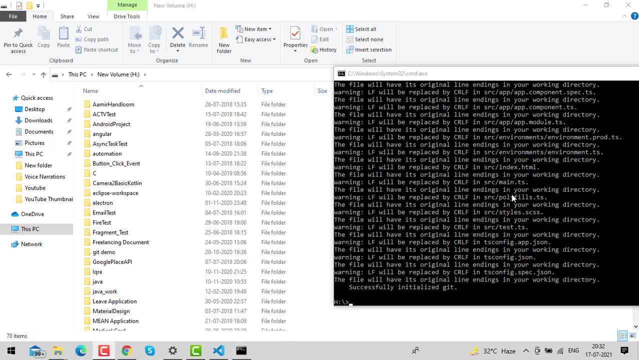 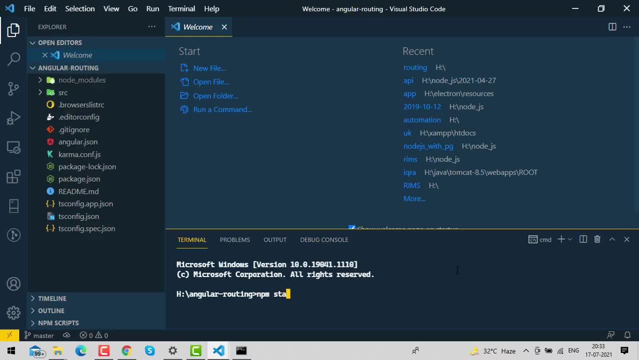 and folder and it will install all the dependencies. So, everything installed successfully, Let's go inside the folder CD Angular routing and open code into VS code. Now let's open terminal And let me start this project. first, Would you like to set this? 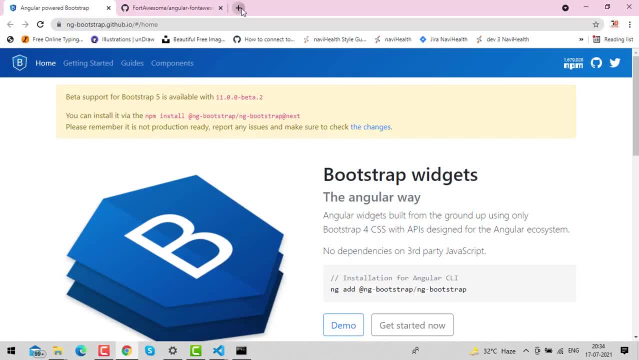 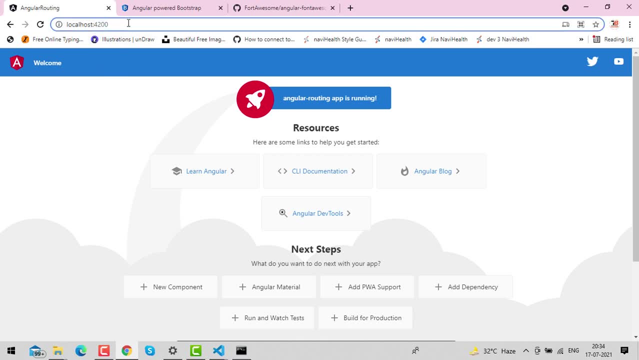 No, as of now. so application compiled successfully. Let's check in a browser, Port 4200.. This is a default port of Angular. Now here you could see Angular application is working perfectly fine, So let's go to the code. So inside the SRC folder you will find app folder And this is the default. 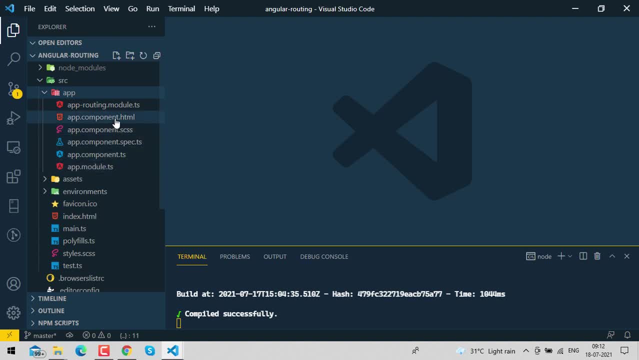 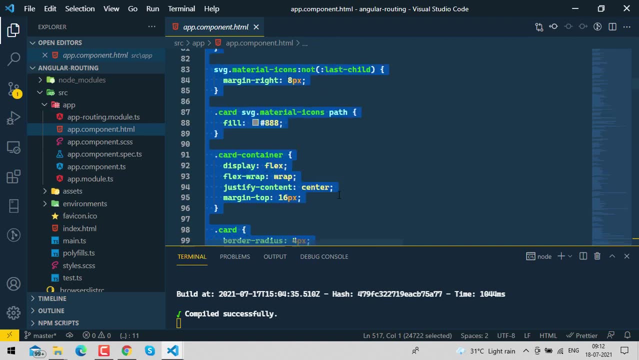 component and app module. So this is the default module. So our application start from app component. So inside the app component you will find the application start from app component. So inside this you will find some boilerplate code. Let me delete all this code And it will go at the bottom. 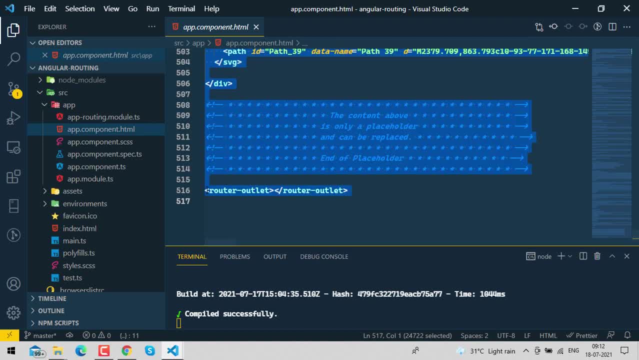 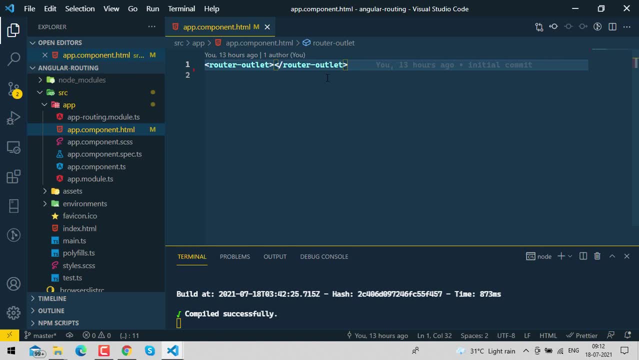 of this You'll find one router outlet. Let me keep router outlet and delete everything. So router outlet is a placeholder where are all the component will render based on router state. So if I'll go to this last login page, login component will render here. If I'll go to forget password anywhere, 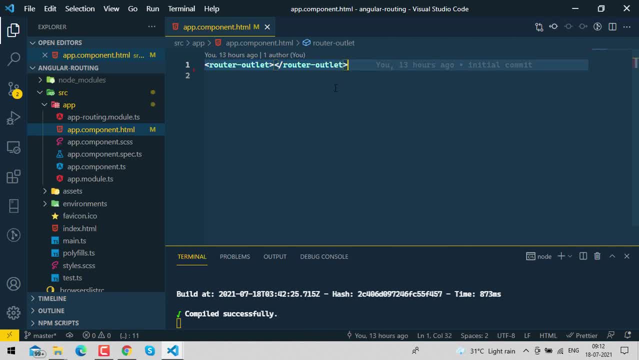 that component will render here. So this is a placeholder. Okay, Now let me create a folder inside app component. I'll keep all the components which belongs to app module inside this folder. Now, inside this I want to create first login component. 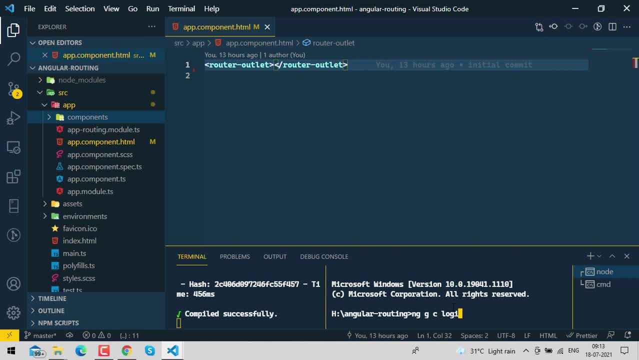 ng generate component login, but it will be inside components slash login, So login component created inside this. So here you could see that this is the login component. So let's go to the app component. See, so this is the login component. Let me create one more component. Forgot password, So I have two. 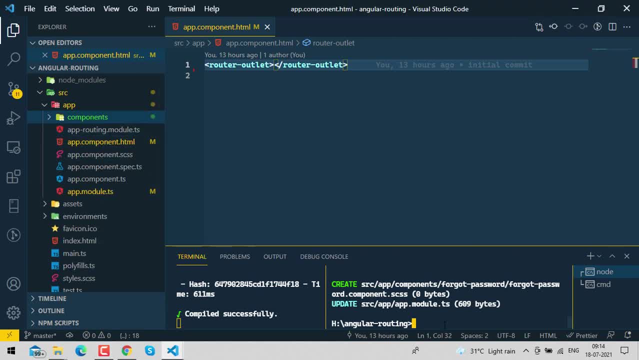 components inside this components folder. Let me create one more components not found, So this will: I'll use this component for 404 if that route is not present in our application. So I've created all three components inside this folder. So let me first 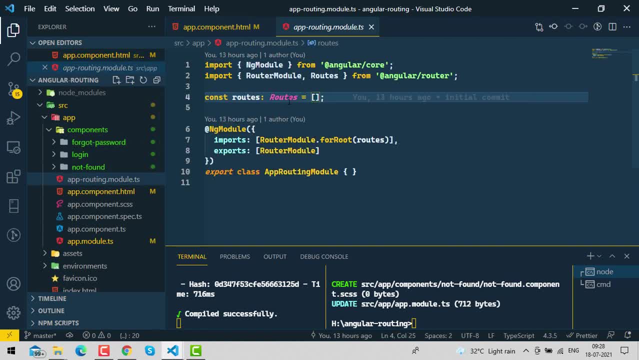 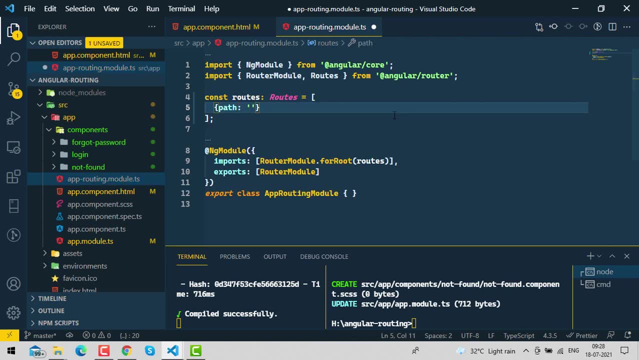 define the route for all these components, then we'll go for designing. So inside this router. here start adding object path. So inside login components. So if user will go to the login component then I want to render login component Okay In a similar. 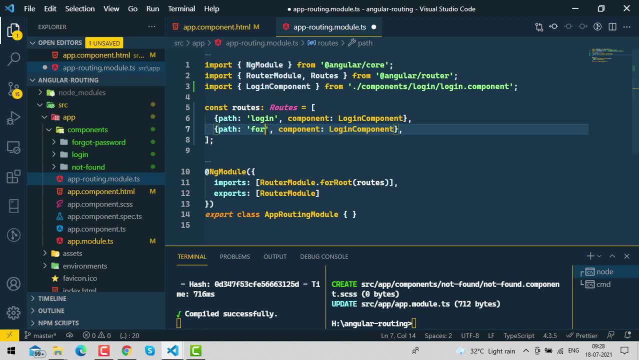 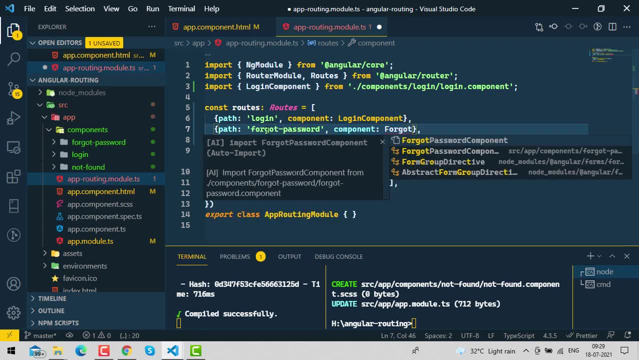 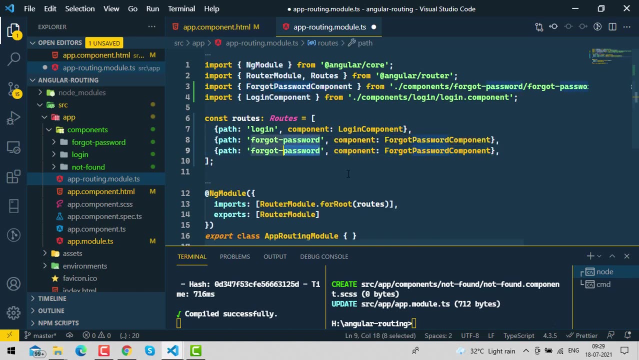 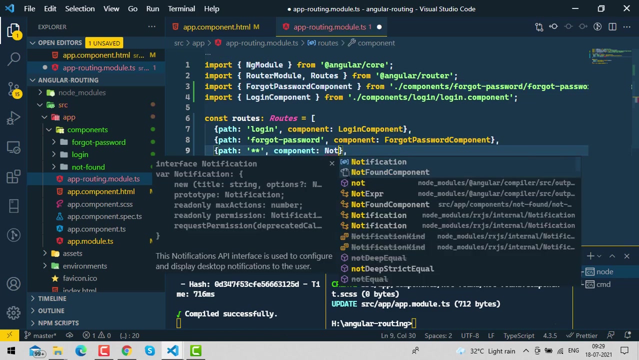 way, I am going to do another, So I actually don't need to run new route. У指跟我 зар toil hacemos再 по н maths созеция not found that we use asterisk and we'll take them to not found component. so I've designed, defined all the routes us to not found component, so i've 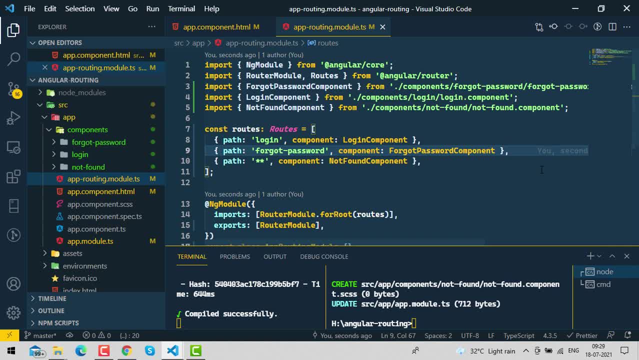 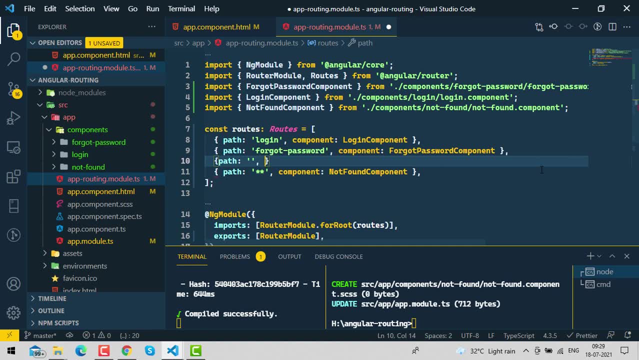 design. I've defined all the routes, So now let me define one more thing. I am going to дела into one of these options I have if I am going to use any different routing tool whenever I am going to run all of this. so now let me define one more thing. if there is no route, present path. if blank, redirect to. 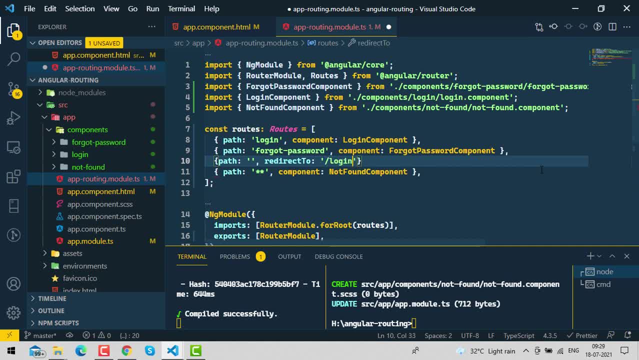 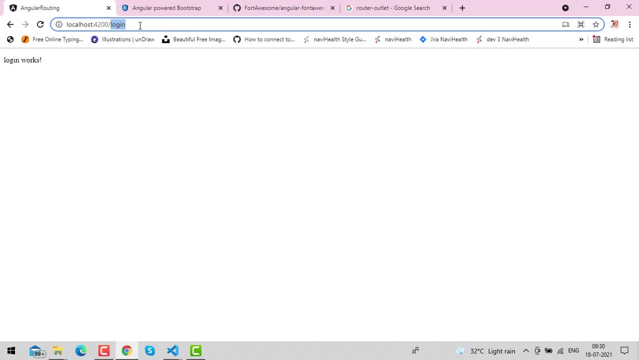 slash login path match full. let's put semicolon. so i did all these things. now let's check in the browser. so by default, if i'll go to the blank route, it will take us to login route. login works here. now let's go to forget password route. forget password works here. if i'll go to any route. 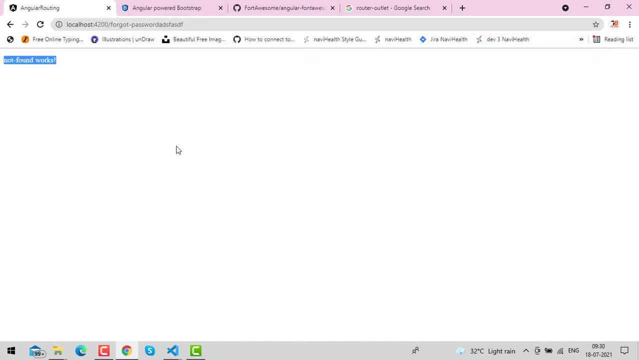 which is not present, then it will take to not found works here. so our routing is working. fine, let's design first, then we'll go for next. for ui designing, i'll use bootstrap and font awesome. so these are the two different packages i'm going to use in this project. 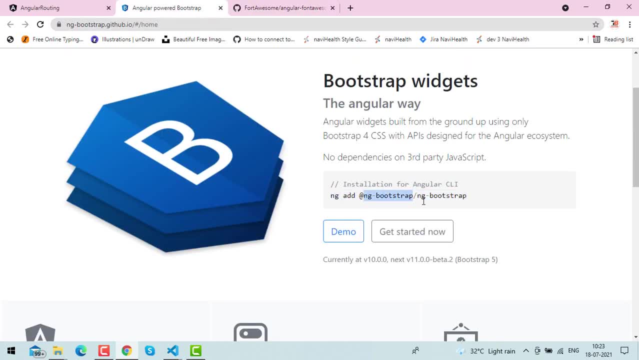 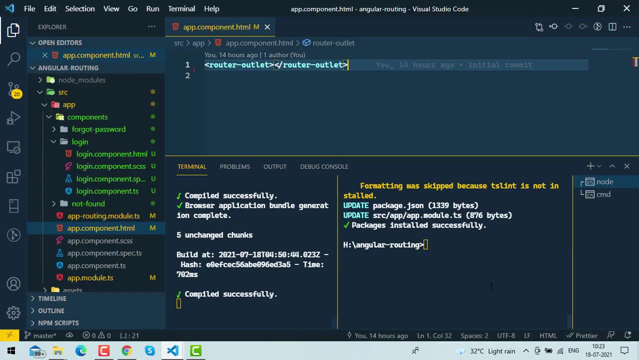 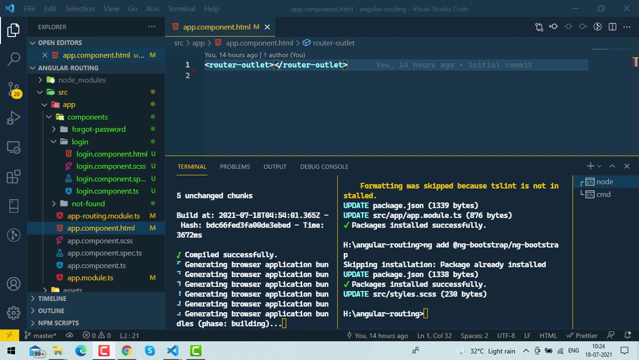 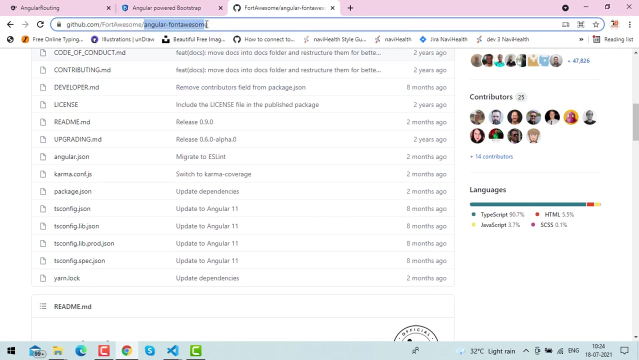 so let me install one by one. so here i'm going to use ng bootstrap. this is especially designed for angular bootstrap. okay, so let me add this dependency in my project first. so ng bootstrap installed successfully. now let me add another package font- awesome. and i'm using angular font- awesome. this is also especially designed for angular. 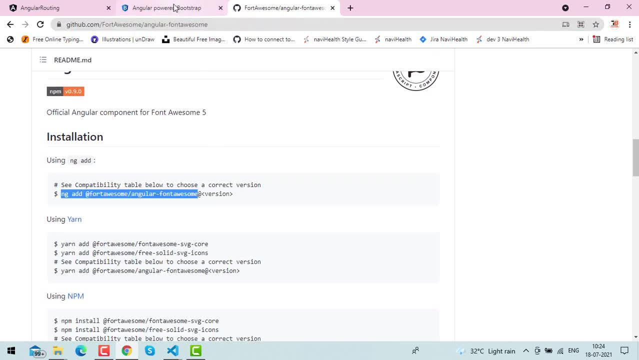 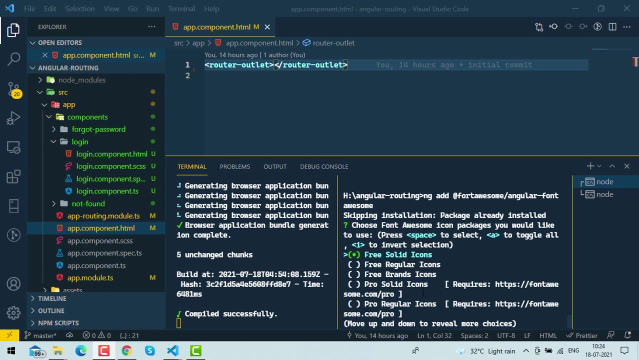 so let me copy this and i'll give the both of. i'll give the both of the link in the descriptions you can check out. let me add these also in my project, so it will ask for options like free solid icons. i'm going to use these free solid icons. 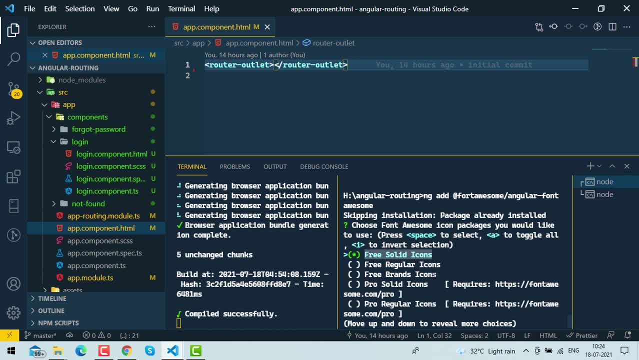 and if you want for some icons, like for facebook, youtube, twitter icons, then you need to install these as well, so you can choose both the options, but as of now, let's go with the default options, because i need only solid icons. both the packages installed successfully. now let's. 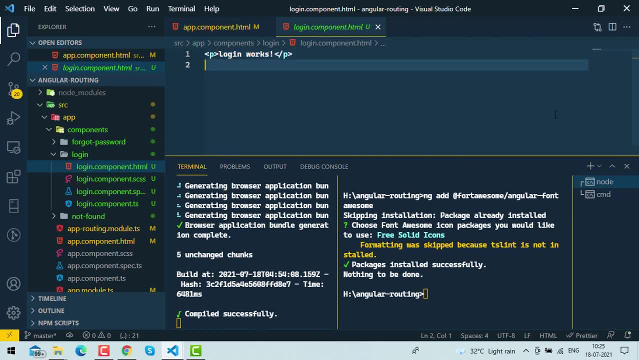 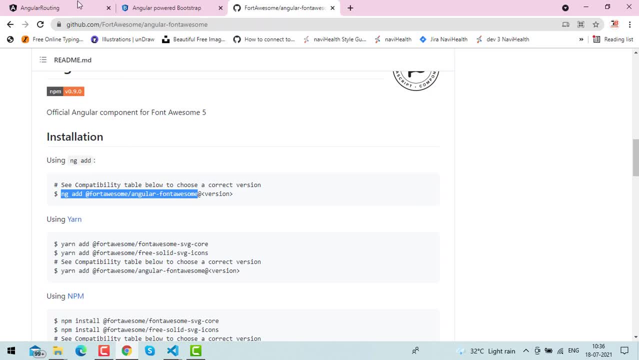 design login page first. so, as i said, uh, this video is not about this video, so let me explain you more about this today. you can see, ok, so let's start with the first step of writing the code here. this is my login page, login page, and there are some. 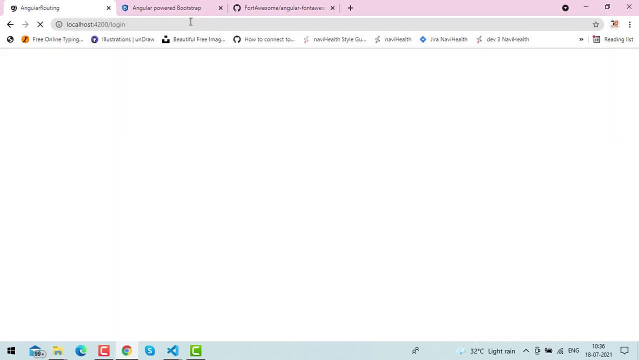 functions are support, okay, so all of them are not in this code. i'm just going to copy paste all the code here. so this is the code for login page. let me save this now. let's go back to the browser and see. so let me go to the login route first. 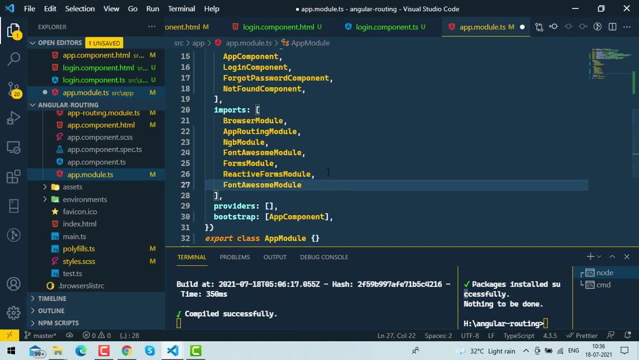 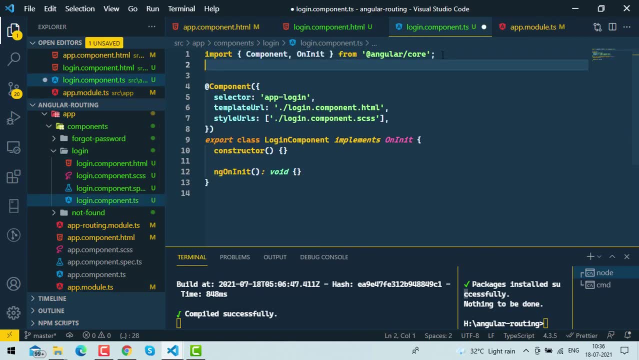 so here you could see this login page is working. the only thing is missing here is log icon. so let me add font awesome lock icon here. login componentts file. here we need to import fa lock icon. so i'm importing this from free solid svg icons: fa lock. now let me assign this into a variable so that i can use inside my template. 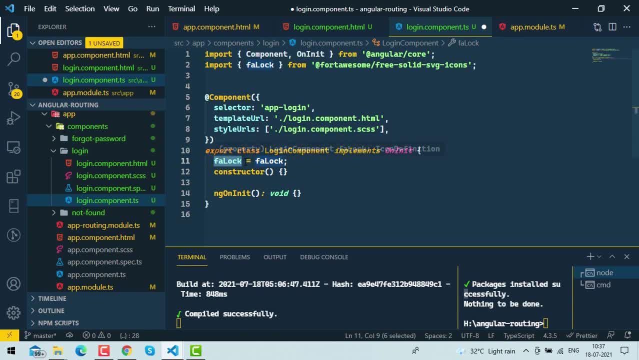 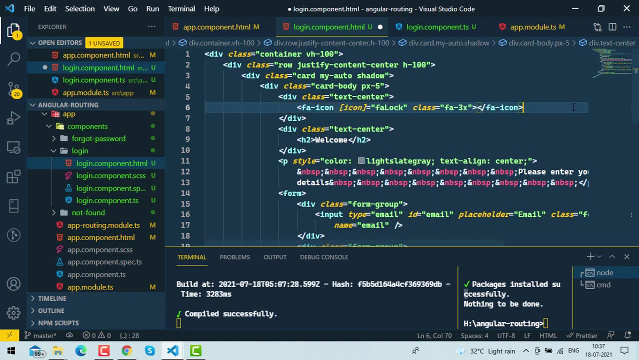 so fa lock icon. i'm keeping the same name so i can use this variable inside my template. so let's go to login componenthtml file and here let me uncomment this, and here you could see icon: fa lock icon. so this variable i'm passing here, and fa icon. this tag only works when we will add. 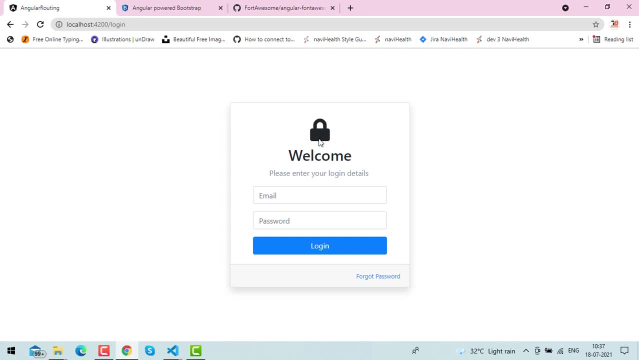 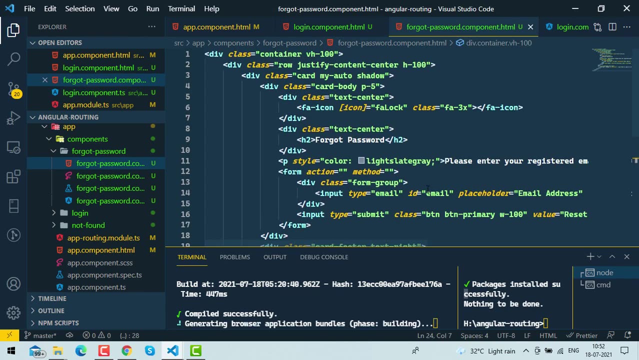 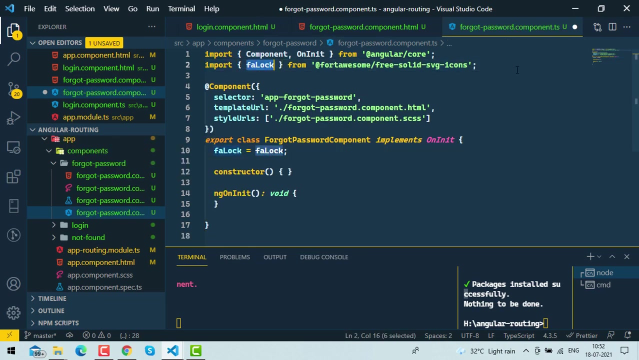 that module: font awesome module. now here you could see. this icon is coming. so now let's go to forget password. component inside html. so this is the code for html. here also, we need to add font. awesome. so we imported this. now it will work as well. now let's go back to the 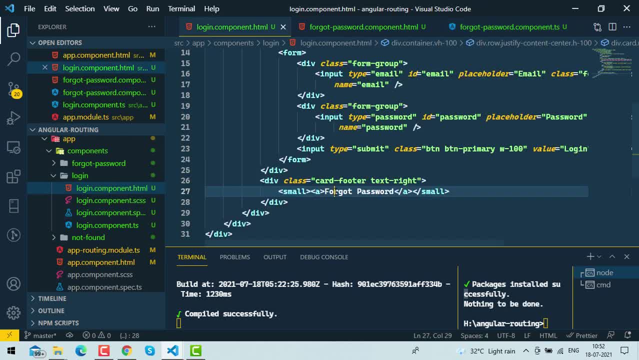 login component now here. when user will click on forget password, it should render forget password component now in angular. we don't use hre for navigation, we use router link for navigation from one view to another view. now here i will specify the path for forget password component. 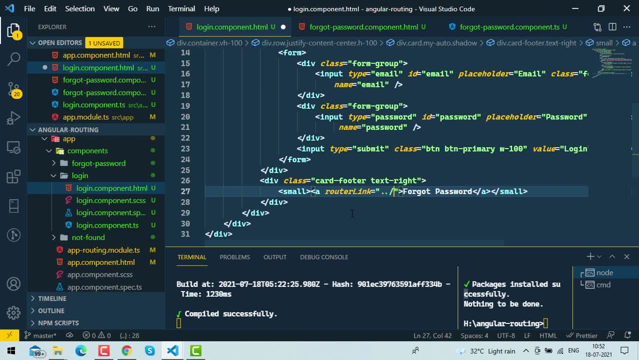 so double dot means we'll go one up from the current path. so current path is slash login, so we'll go one up and then we'll go to forget password path. so here, forget password. okay, so that's all. now save this and check in a browser it's working or not. so i'm inside login if i'll. 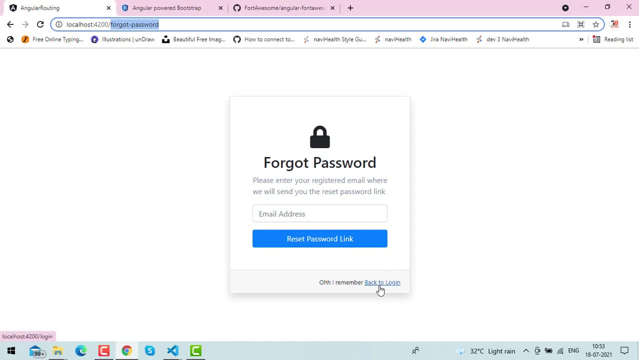 click on forget password, it's redirecting to forget password path. okay, in the same way i did for the back to login option. if i'll click, it will redirect to login page. now it's working fine. now one more thing left in app module. i haven't done any designing for page not found. if user will. 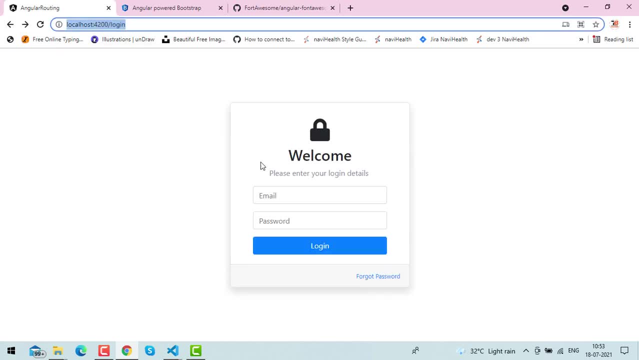 go any route which is not present, so let me design this page first. 404 not found. so let's go to the code and here also i'll do the copy paste now. save this like this so it will take us to the page not found: 404 not found. here is a button in this. 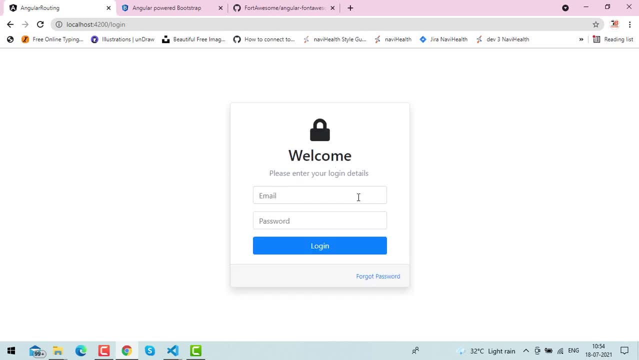 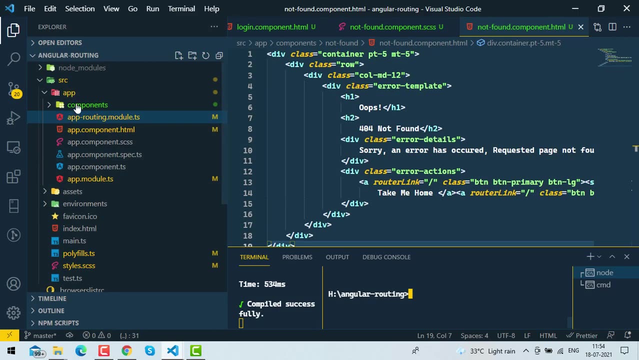 button. also, i add router link and it will redirect to the login page. so now let's understand lazy loading and protected route using auth guard. so let's go inside the code and let me create one more folder inside app modules. i'll keep all the modules inside this folder. now let me generate one. 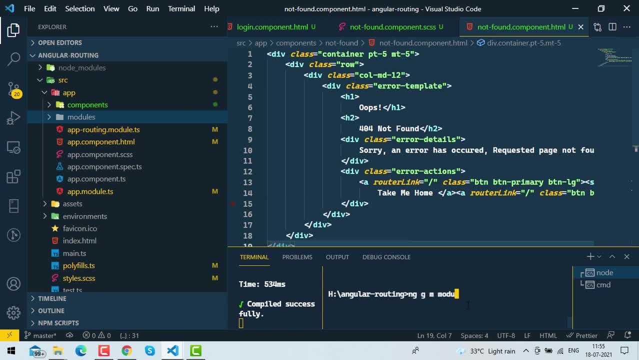 module ng: generate module inside module folders admin and also i want routing, so add the flag hyphen, hyphen routing. so this command generated two files: admin module and admin routing modules. so i'll add all the components inside this module and simply can generate a new module and actually 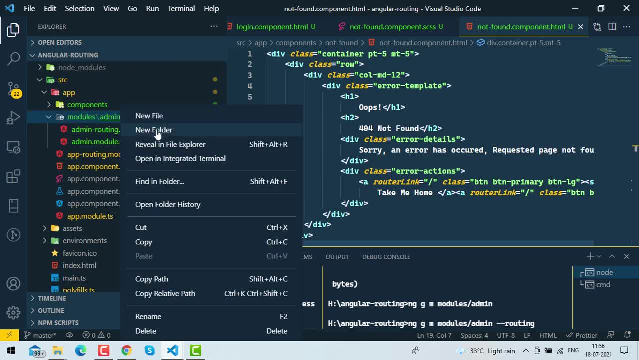 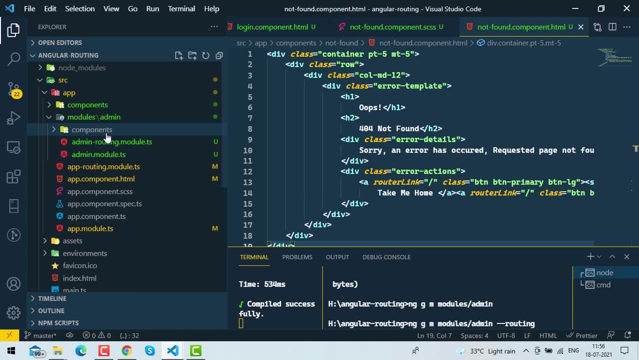 module which belongs to this module. okay, so let me create one more folder here, components. here i will add the default component means admin dashboard component. okay, so let me generate one more component here. ng generate component slash, component slash: admin dash board. now, inside this components folder you could see there is a dashboard folder. so now, by default, i: 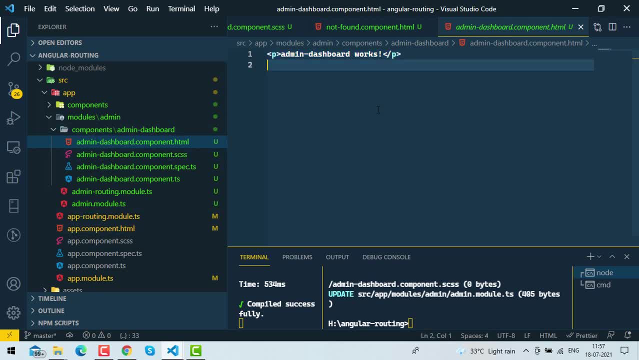 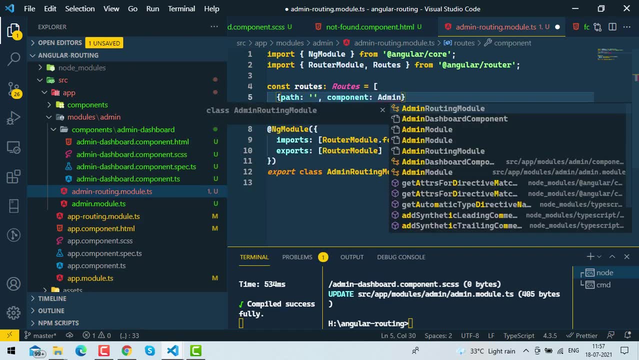 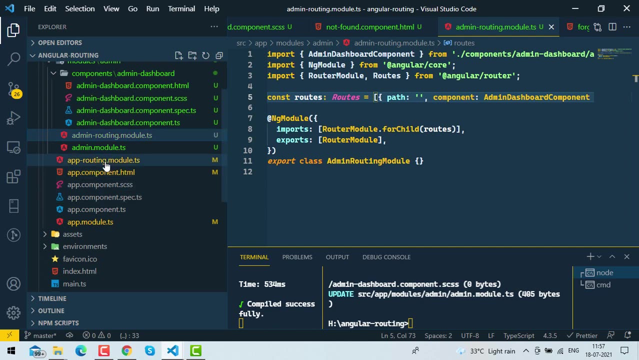 want to load this component. so now let me add routing for this. first inside the admin routing, so in a default path admin dashboard component. i want to load this. okay, now let me add this module as a lazy load module inside a app routing module here: path admin. 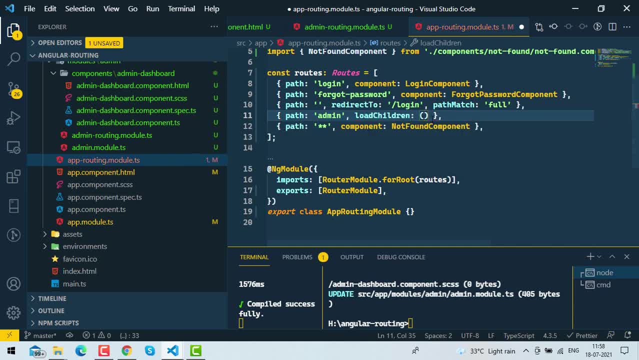 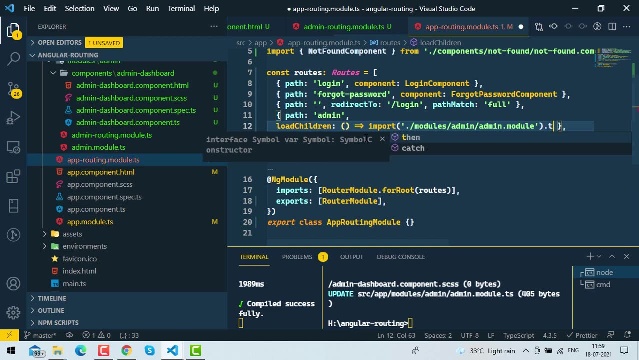 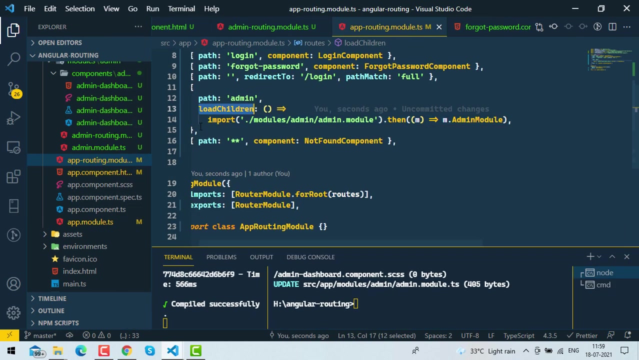 component: load children. this will take a function import module: slash admin. slash admin module. i want to import this. then i need to use dot, then admin module. so this is the way to do the lazy loading right. so if user will visit this route, then only we have to do the lazy loading right. so if user will visit this, 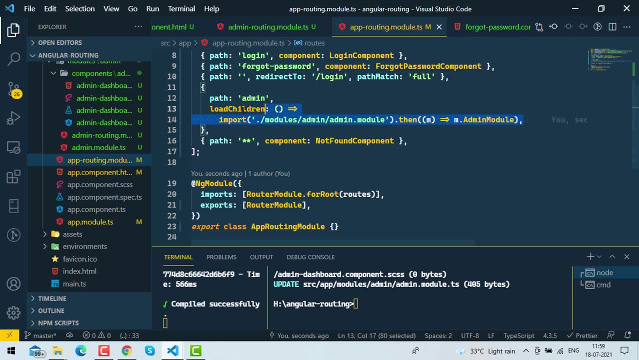 route, then only we are going to load this module. apart from that, at the time of bootstrap we are not going to load this module. so this strategy is used to make application more fast on the demand. only we are going to load this module. now let's see this application is working or not if user 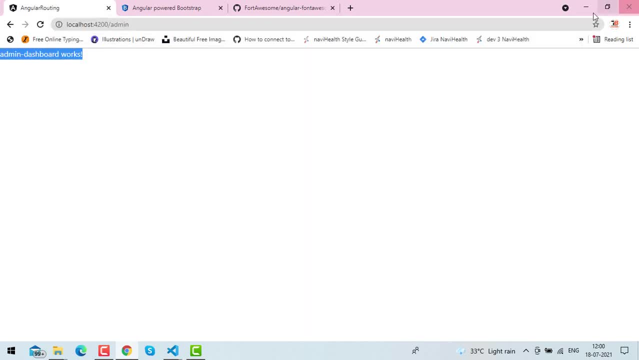 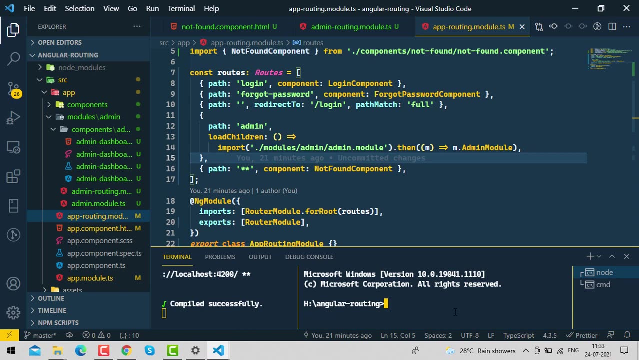 will go to admin. now. here you could see admin dashboard. so admin route. this is also working fine. now let me put: uh. so now let's first create all the components of admin module ng, generate component module tools inside that admin, inside that components, and then we'll first generate header component. 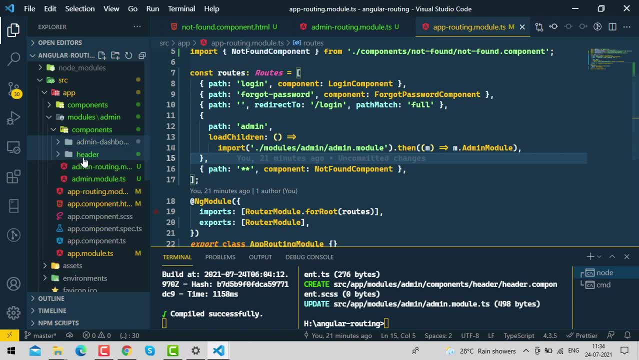 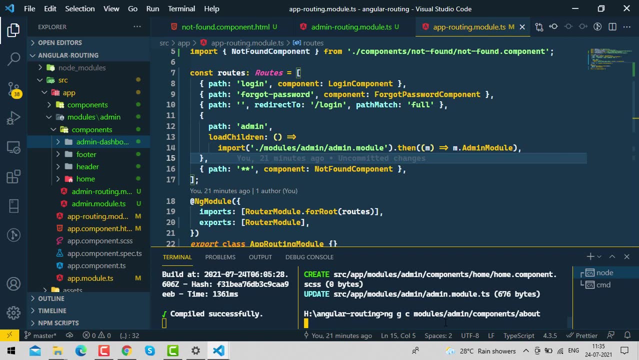 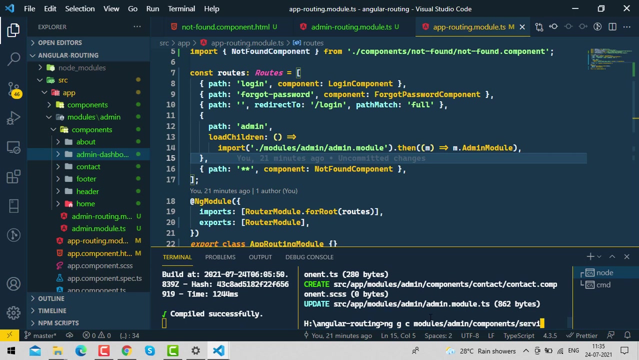 okay, now here you could see that we have admin dashboard and headers in the same way, let me generate all the other modules, like footer, as well. now let me generate few more components, like home, about contact services. so almost all the components i have generated admin dashboard, so this component will work. 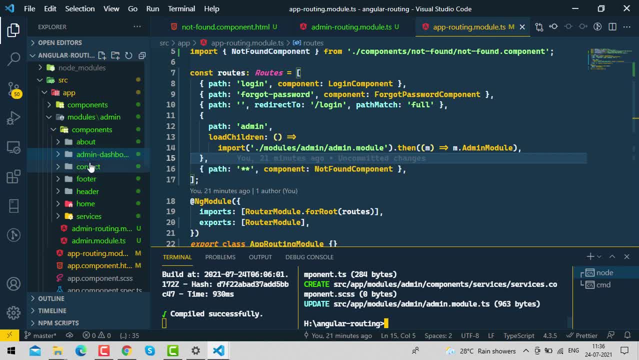 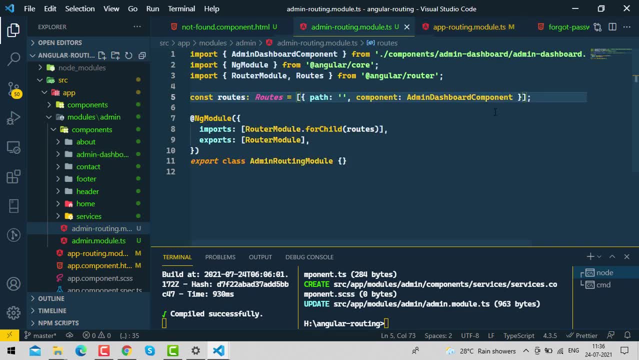 as like a container. so from inside this component we will render all the different components. so hey, let me create the routing for this first, then you will understand each and everything. so this component will become a parent component and all the components which now i have generated like: 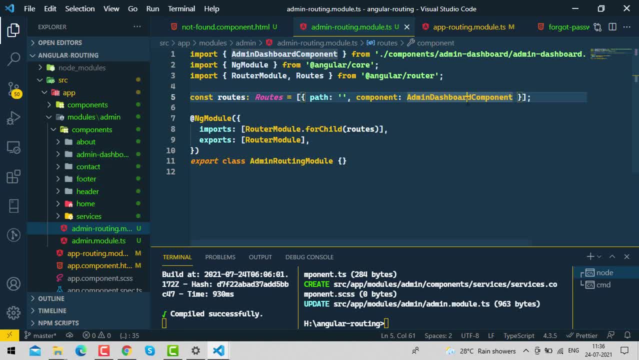 header, like about us, will become the child component of this. so inside this component. first let me add two things. so here i'll add admin header, header component and footer component. i'll keep here and all the other components. so here i'll add three things: header, footer and router outlet. 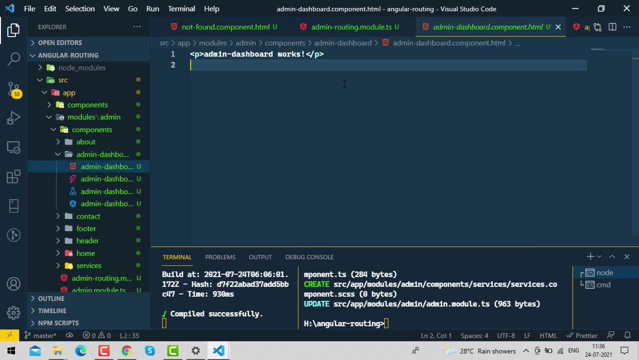 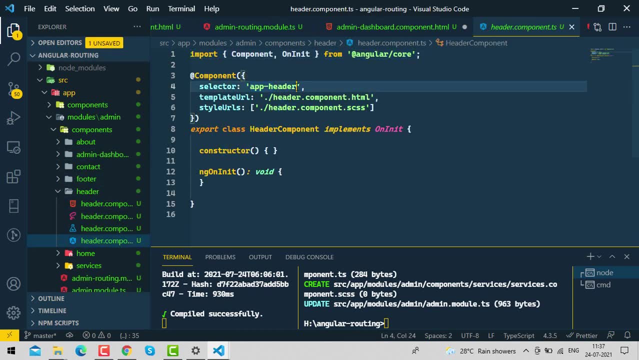 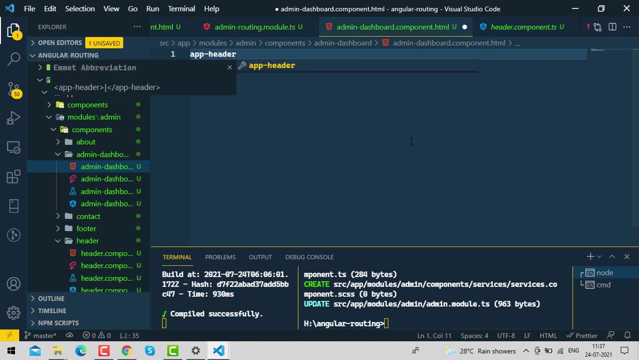 so let's first go to admin dashboard component. so let me let me keep this as of now. go to header. so this is the selector. just copy this app header. go to admin dashboard. here. let me put this as well as a tag so it will render header. here now in the bottom, we'll render. 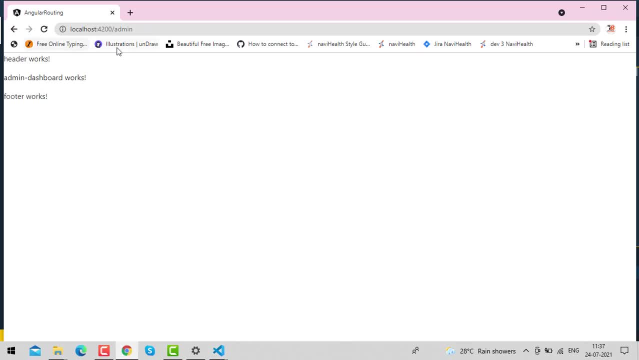 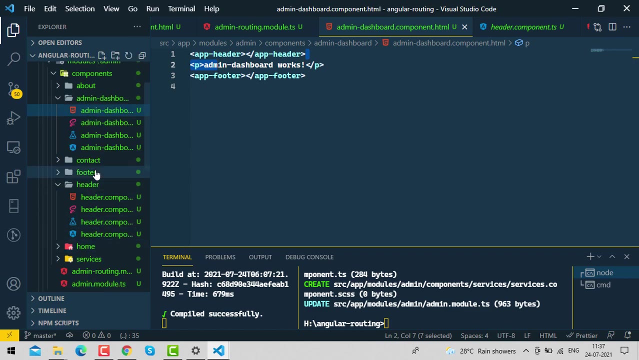 footer. okay, both the things we are going to render. let's first check this. so inside the admin you could see header and footer are working and inside this this is a admin dashboard. okay, now let me define the routing first, then we will design header and footer. okay, first go to the admin. 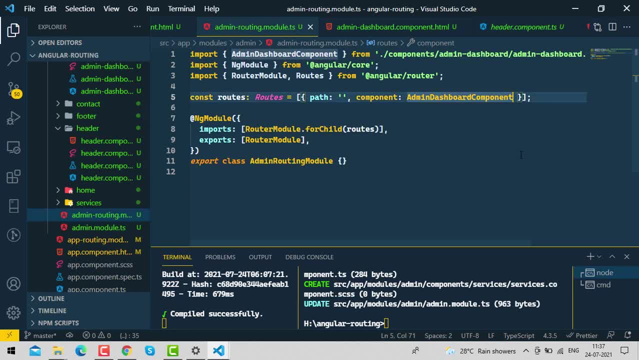 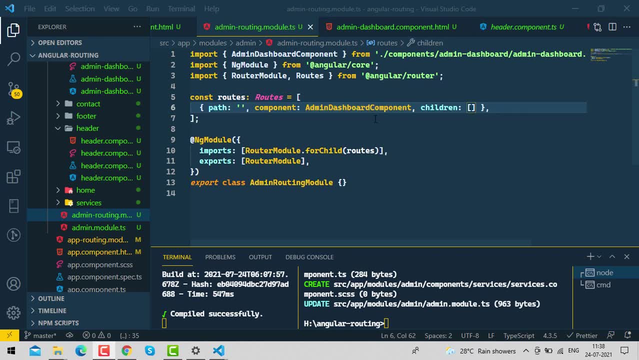 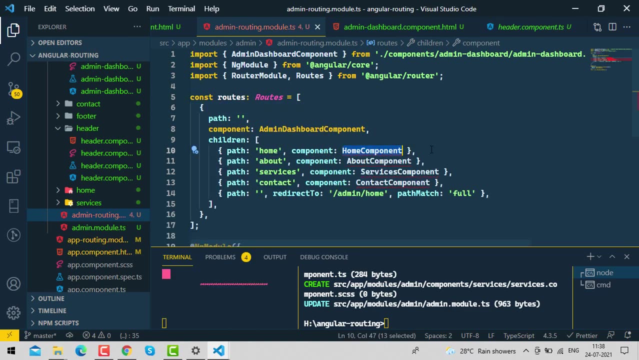 routing module, so admin routing module. in here let's use children. this will take an array and all the different routes which belong to admin module will put inside this children route. so now let me put all the different route so home component. we'll call this home one by one. all the 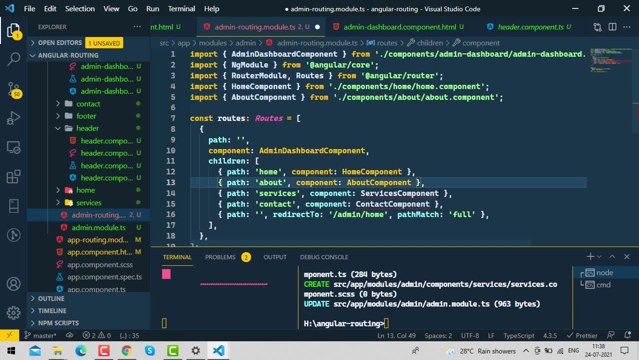 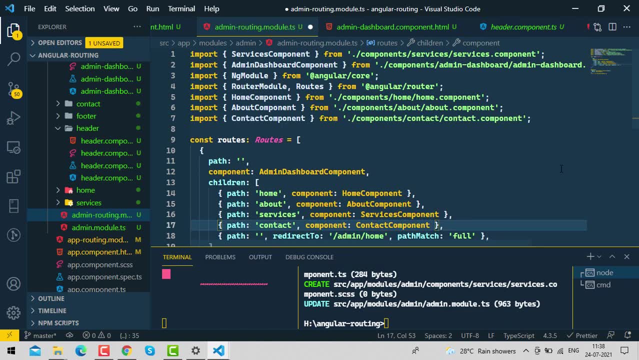 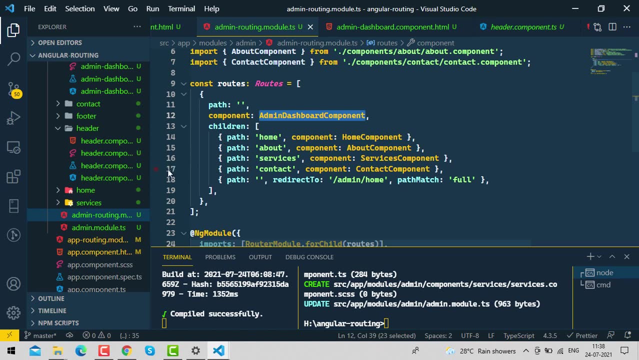 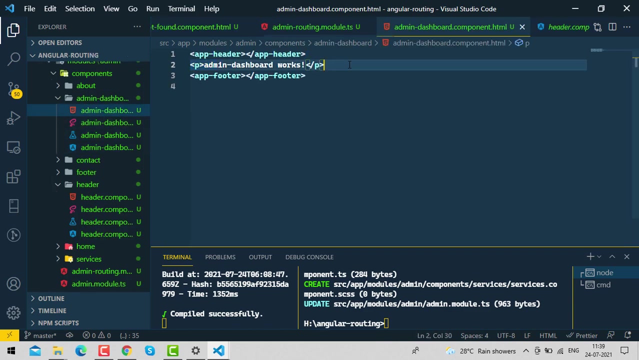 components. let me import component which we have generated, then services component and also the contact components. so now these are the child routes of these component. now, inside this we could put router outlet. a router outlet will not work if you don't have any child routing admin dashboard also. instead of this, I will keep router. 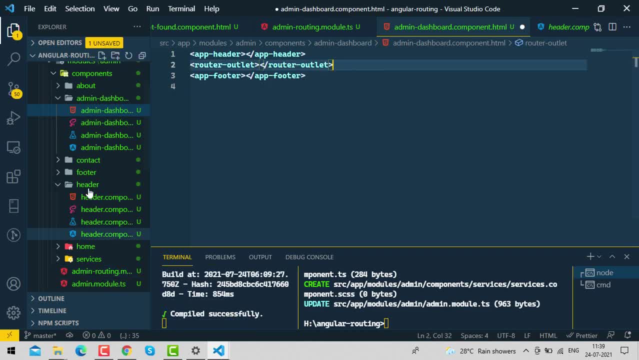 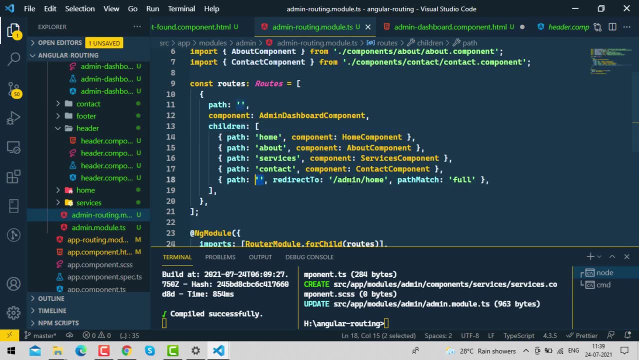 outlet. so what will happen? let's first understand. let's go to the admin routing module so, as I have already redirected, if there is no route match, then it will redirect to admin home and if we'll go in any other route, then it will go in these routes, but by default. if we are in inside in slash admin, then 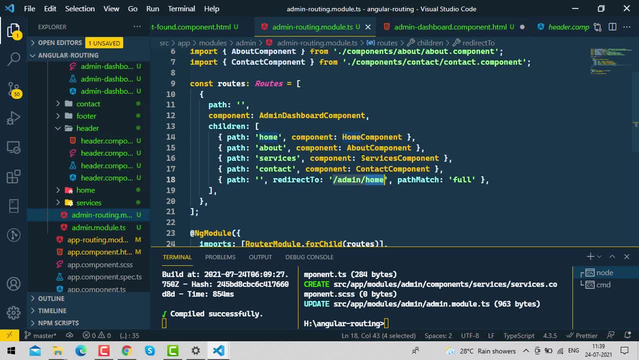 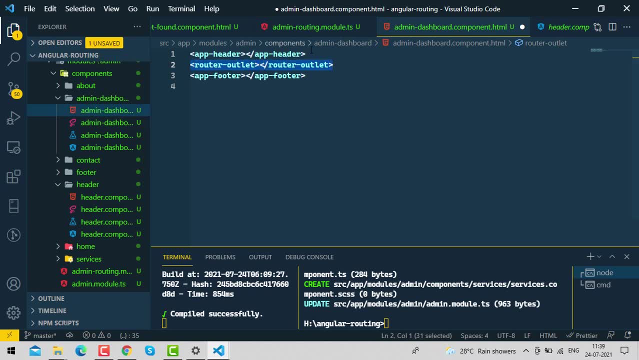 it will redirect to slash admin, slash home. okay, now where this component will render. this component will render inside admin dashboard, will render here, and header and footer will be common in every route. oh, because we keep the router outlet in between these and these module will render inside app component. 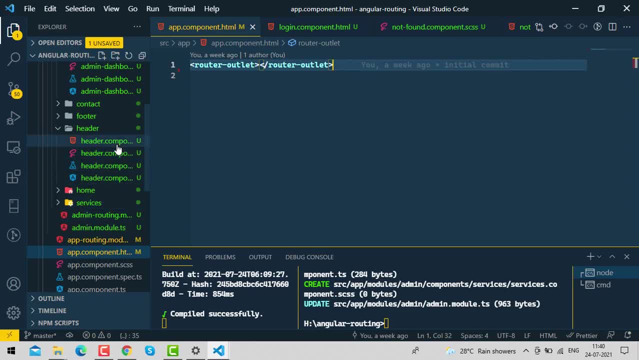 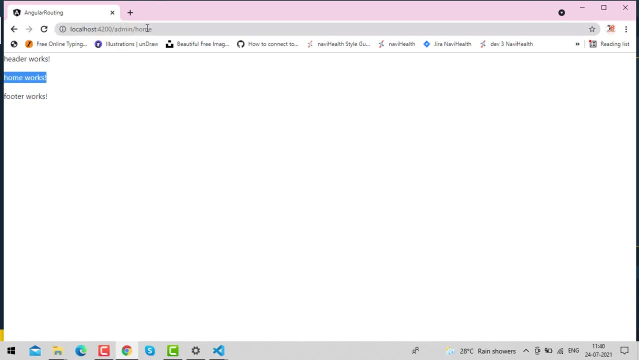 right, it will render here. so now let's check in the browser first. in the browser now. here you could see: by default, if we'll type only slash admin, it will redirect to slash admin, slash home, and here you could see home works. now let's go to about. here you could see about works. now I will go to services. 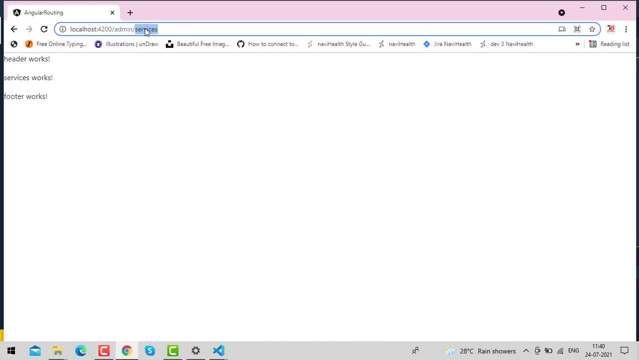 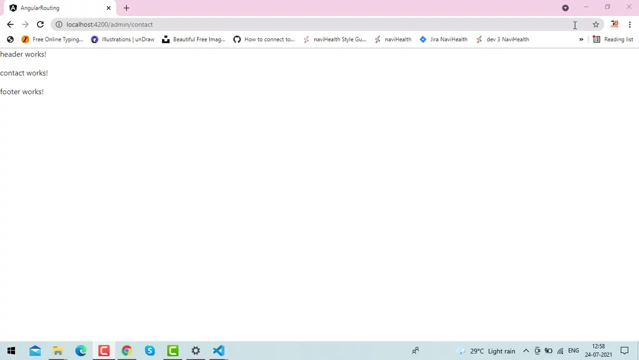 here you could see services works and if you'll go in contact, see contact box. so all the routes, here it's working perfectly fine. now let's first design, then we will implement auth guard and other things. now let's design header first. so let's go to the header. component of admin module. 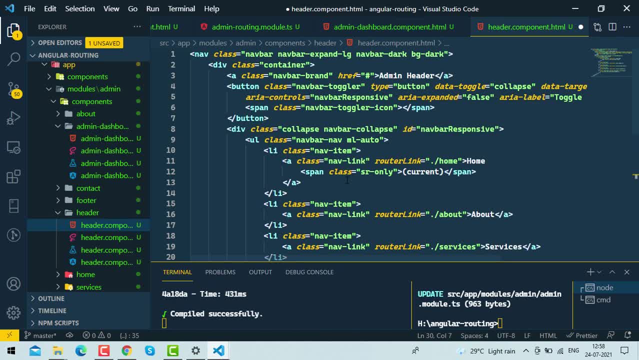 now here let me paste the code. so here you could see i created many link and in all the link i use router links. so, as i already explained, router link we use instead of href in angular. so if user will click on home will redirect to dot slash home from the current path. so the current path is. 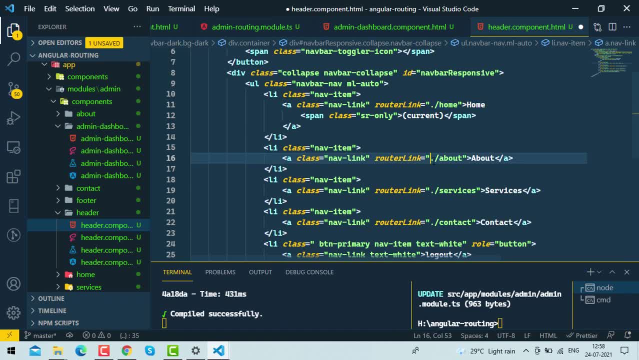 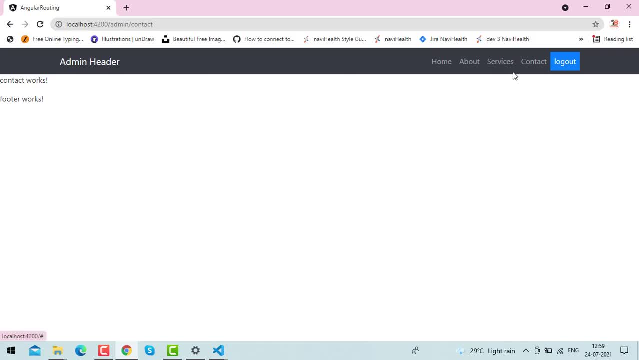 admin. so we'll move to the admin slash home admin slash about admin slash services. so in this way i design. now let's save this and see the output. so here you could see header component. so if user will click any of the link, if i'm clicking i'm going about us component, but we have a common 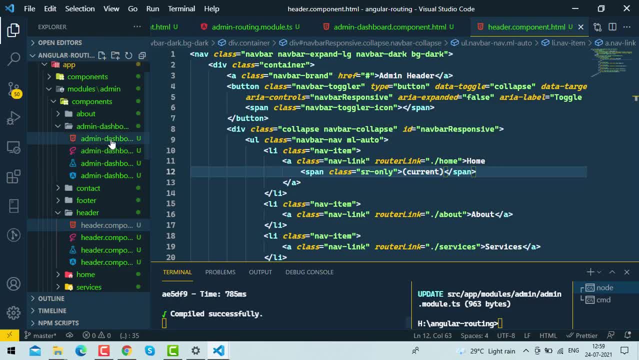 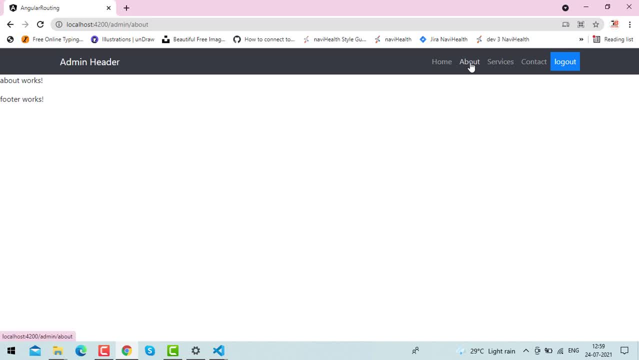 header. only the body part is changing because of in admin dashboard we keep router outlet in between and header is common in all the routes and if i'm clicking anywhere i'm going in that routes. okay, here we put the services change, contact change. if you have noticed one thing, if i'm clicking on any 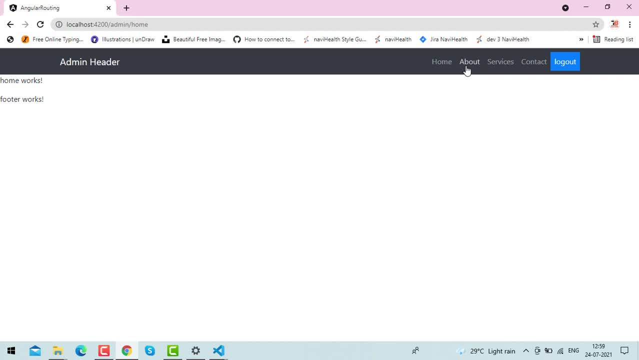 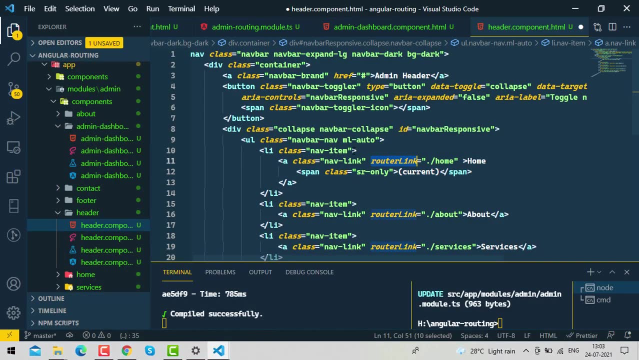 of the services. it's not activating. okay, it's not active. it should be active. it should be in white color, so for that we'll use one more thing. so let's go in a code. we have one more router link active, so this directive will add active class into this li tag once this link is active. 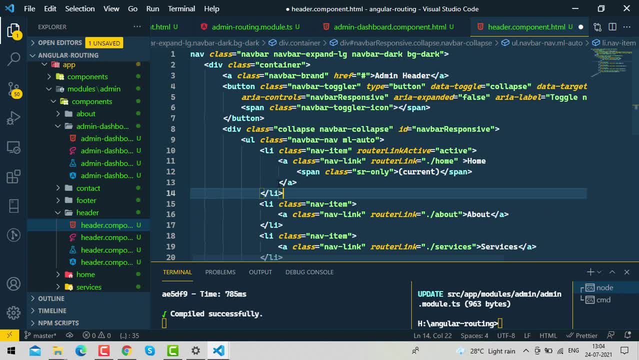 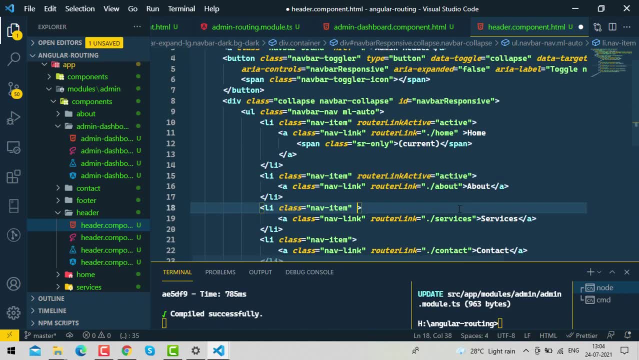 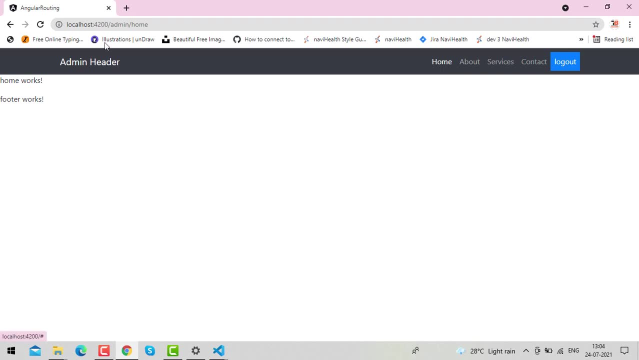 so once this link is active, then only this class will be added to this li tag. so in the same way, let me add this in every places, every li tag. now let me save this so here you could see home is by default coming on. white color means home link is right now is in active link. okay, now, if i'll go, 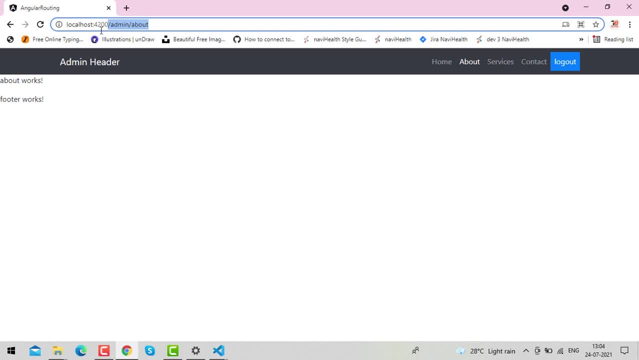 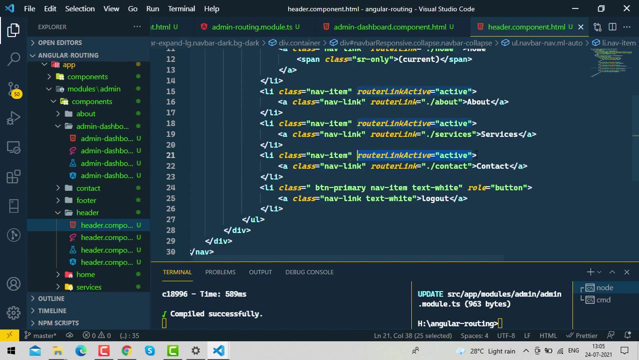 to about. here you could see i'm at about route and here you could see about is also active in white color. so white is coming from the active class. so we are adding and removing this dynamically through router link active. if you get a situation, then you can, you could use this router link active. 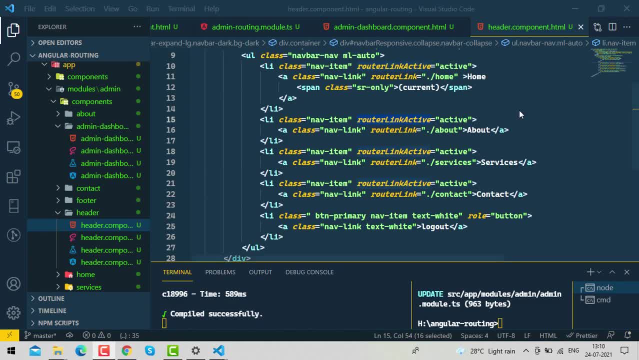 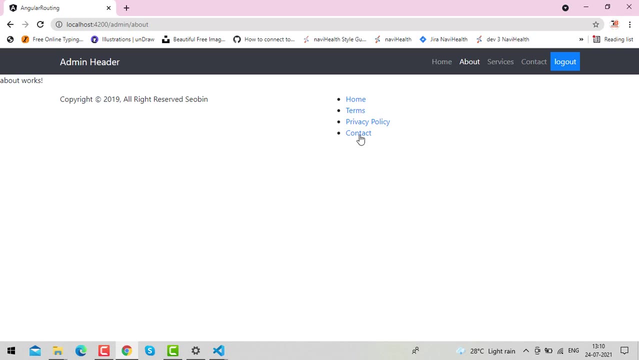 for activating, for adding or removing any class in your link, and remember these are css class. you can add or remove any css class using router link. active now. let me design footer. now save this. let's see, so footer is coming here, but there is no design. let me add all the css. 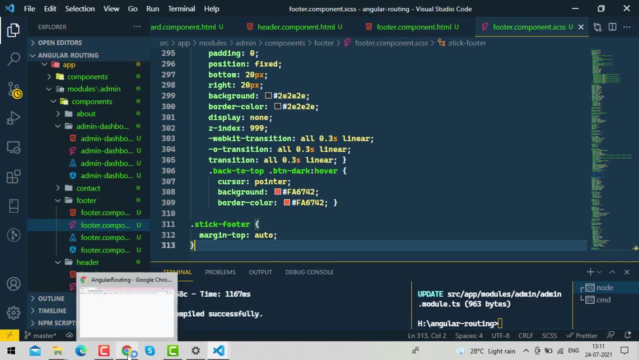 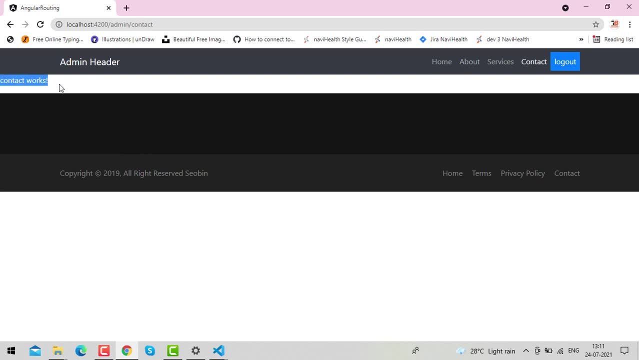 for the footer. you can get all this code from my github account, don't be worried for that. so here you could see, footer is also coming. and in between, all the components. now let's design all the bodies, all the component about home services and contact. now let's design first about component. let me 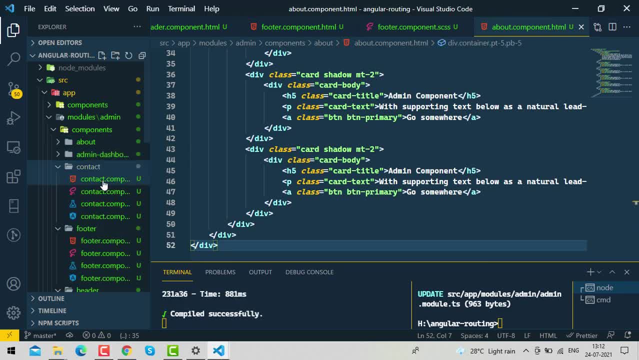 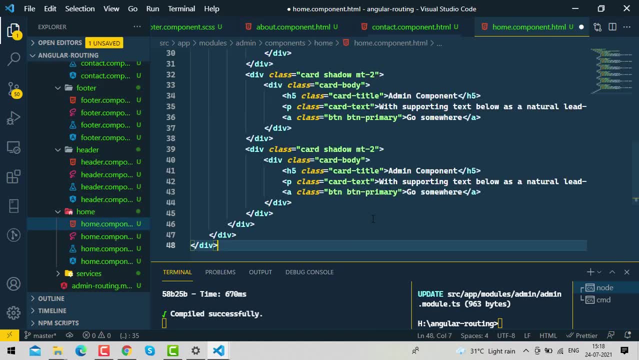 paste the code here. in the same way, let me design contact. save this, then go to footer is already done, header also done. let's go to home. in the same way, let me design home as well, then services. so design almost done for every component. now let's 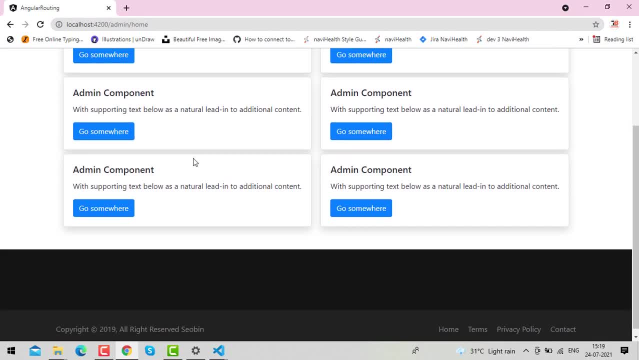 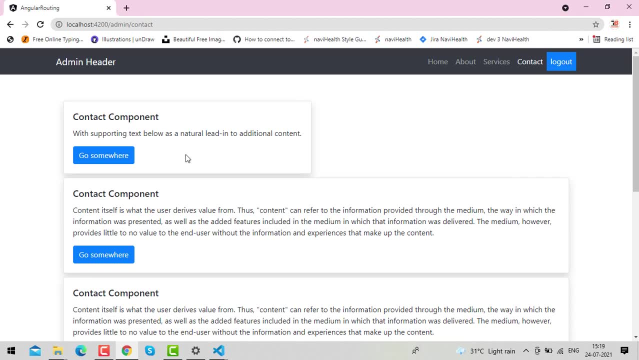 check each and everything is working or not. so if i'll go in the home component, you could see the design in about. you can see also the designs services contacts. for the designing i just use bootstrap and normal css. very few thing left in this video like i haven't written any logic for. 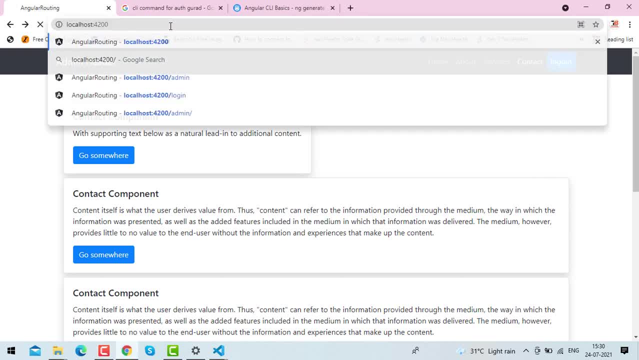 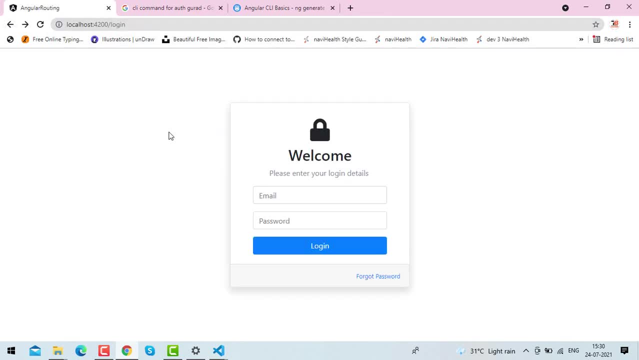 logout and apart from that, i haven't written any logic for logout and apart from that, i haven't protected this route. so any user without login also can come to the admin route. let's take an example: without login i could also go to the admin, but what i want? only the logged in user, or? 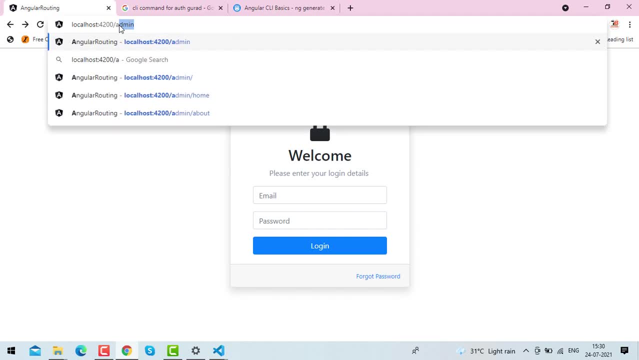 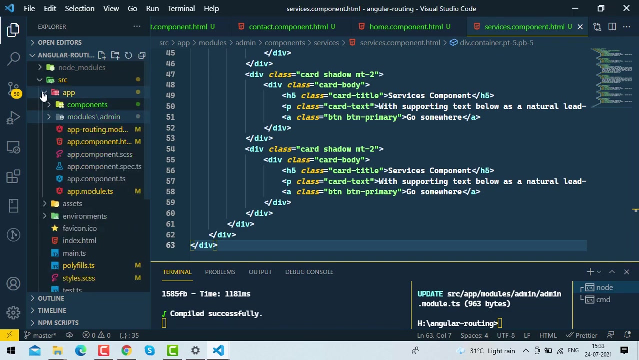 authenticated. authenticated user can go to admin route. apart from that, we will block this route for the access. okay, for this we need to implement- can activate guard. so now, let's do this. now let's go to the code. so, inside this app folder, i want to create one more folder. 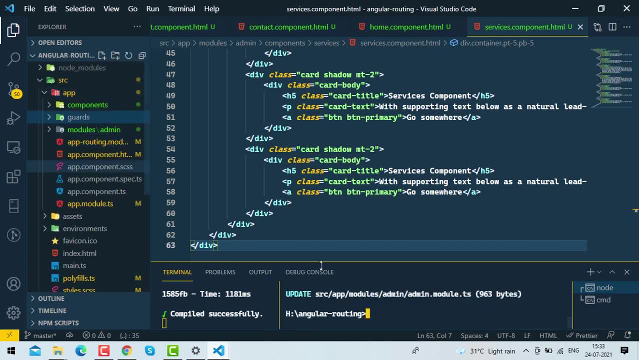 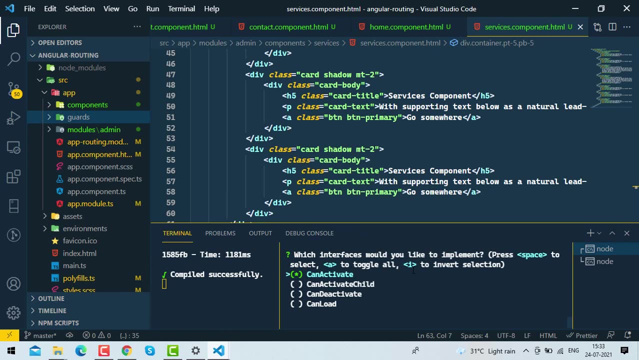 guards. so here i'll create one guard ng generate guard folder. i'll create auth so it will ask few questions like which guard you want can activate, can activate child and deactivate. so first of all i want only can activate, so just hit enter. so if you'll go inside the guards you will find one. 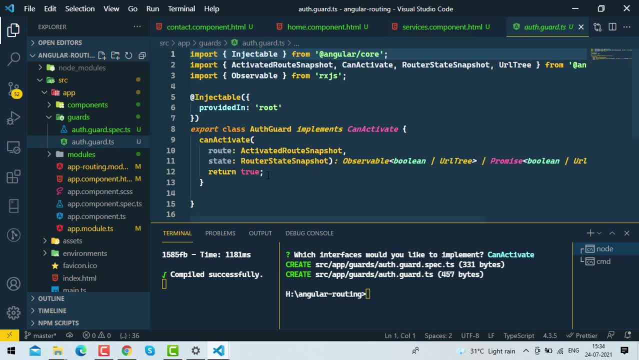 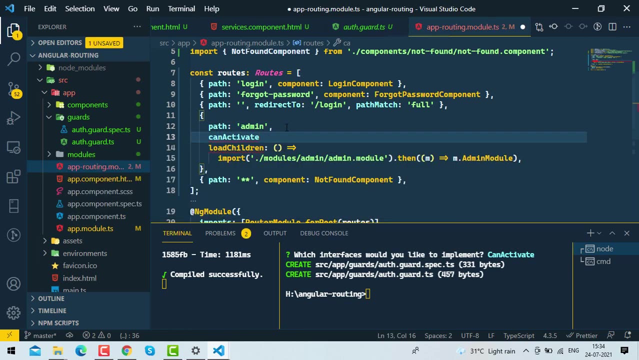 auth guards. so this is the guard i want to implement. so from here, if we will return true, then only that route will be activated. otherwise that route will not activate. where we will place this guard? so first let me place this guard, go to app routing module and here can activate. so here we will apply guard inside an array. let me import. 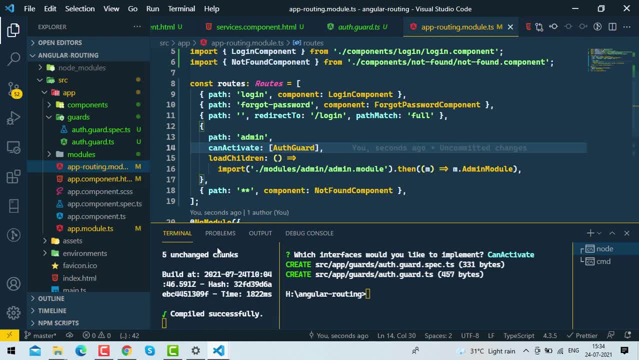 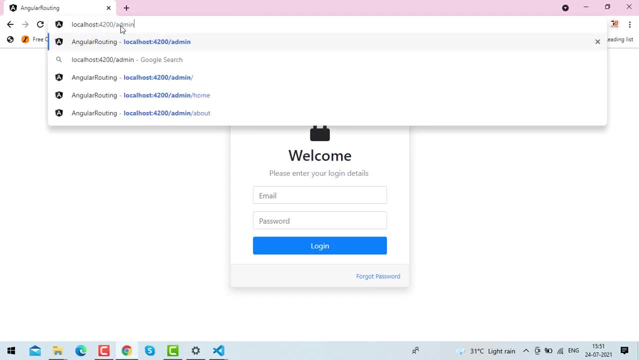 this guard put semicolon. so we implemented guard so we can access this route. we can go to the admin as of now because we are returning true from that guard. if we will return false, we can't go. let me show you that. save this now. if we will try to go to admin, we cannot go to admin, right? 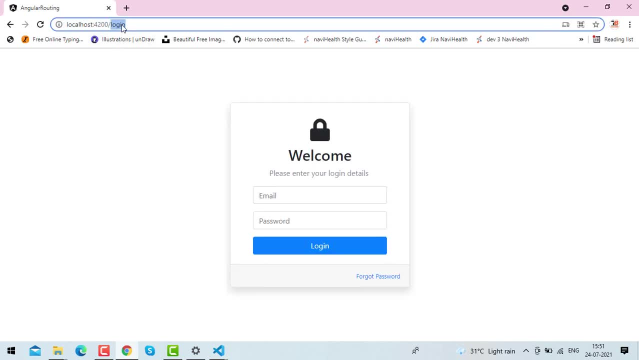 so we are blocked, we cannot go to admin. but if you have noticed one thing: if you are trying to go to admin, the blank page is coming because we haven't written any logic for false. if we are returning false from auth guard, then we need to also write the logic for redirection, like 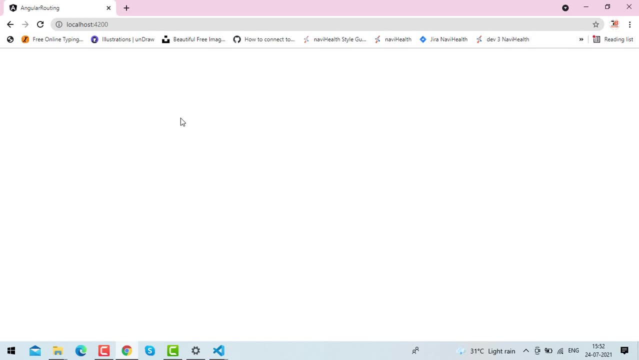 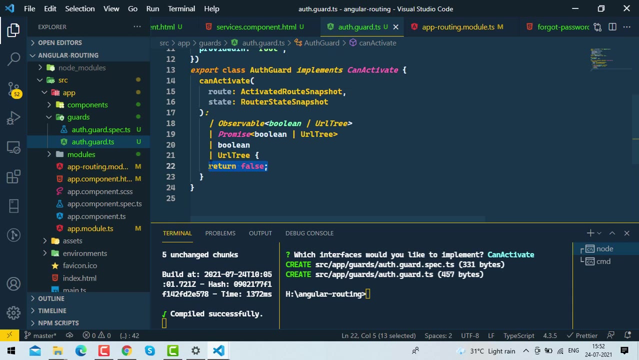 if user is not authenticated, then we will redirect the user to login page. so let's understand here. so all the logics we will implement here. we will check if we are implementing jwt token, then we will check here token is: is valid token or not? if valid, then we'll return true, if not it will fall. so let's implement each and everything. 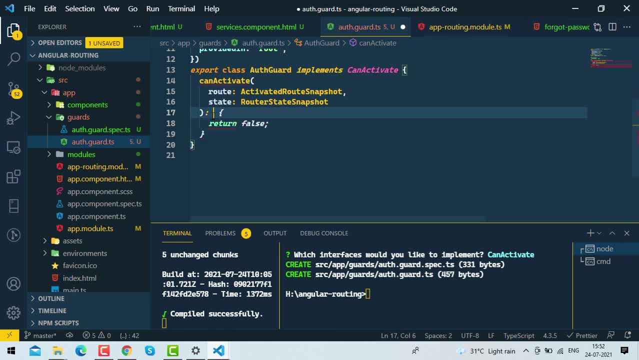 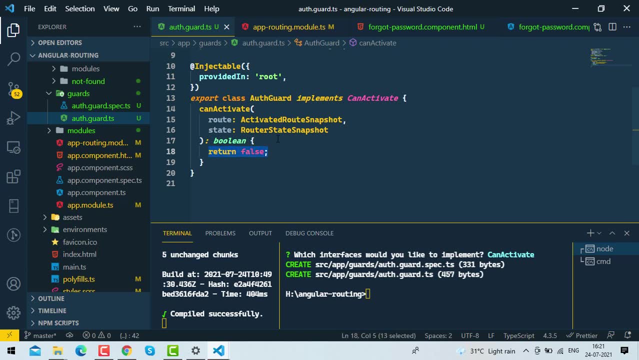 let me remove all the returns, so we will just want to return boolean. so, basically, we are going to return true or false from here, based on authentication. so we will check. if user is authenticated, then we will return true, if not, then we'll return false. so for authentication, let's. 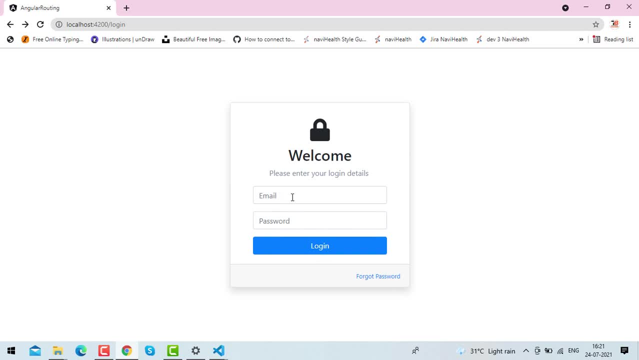 first implement login page functionality. so in normal scenario, what we do? we send email and password to server and server returns either jwt token or a message: invalid user and password. so we will create a reactive form and will implement the logic for this. so let's go to the code. let's go to: 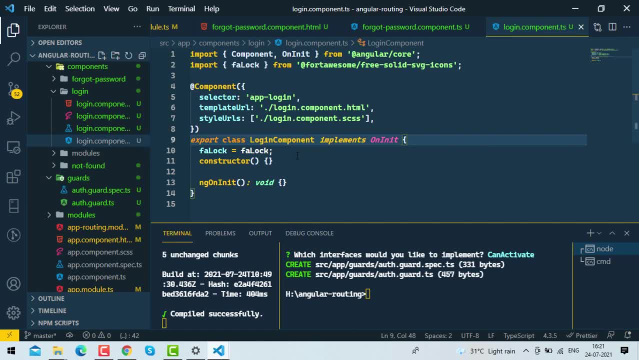 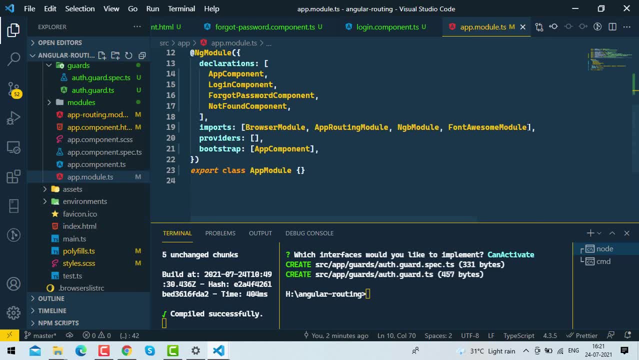 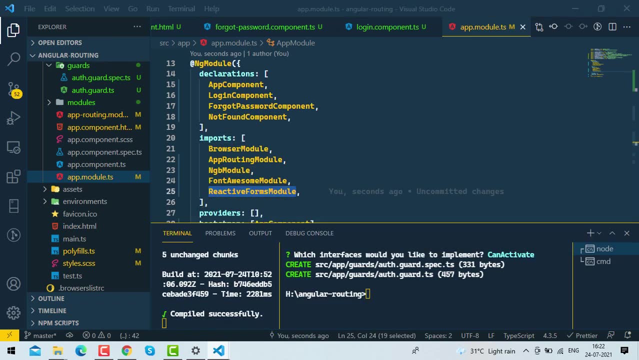 the inside a login page component, and here we will create a reactive form. so reactive form is dependent on reactive form modules inside. go to app module and add reactive form modules, reactive form modules. so i'm i imported that. now i can create a reactive forms. so let's go to login component here. 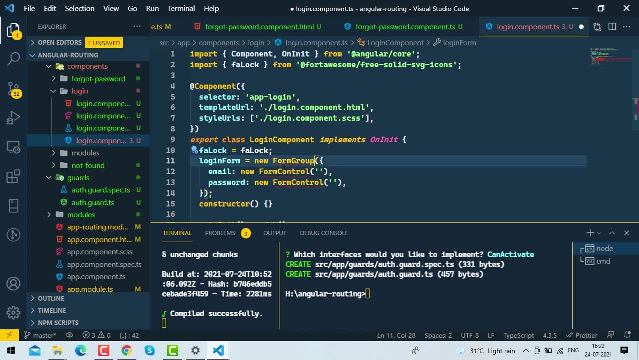 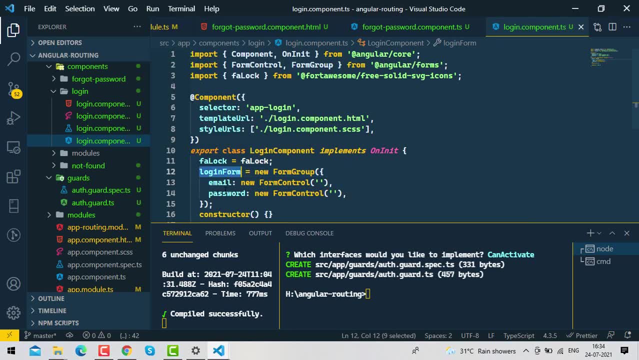 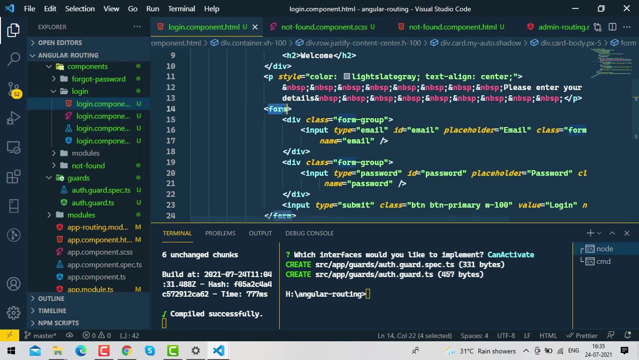 now let me create a. so we need to import first form group class and then form control. so i have created login form that contains email and password. so let me bind this form with my template. so inside the template you will find form tag. so inside the form tag, first we need to implement. 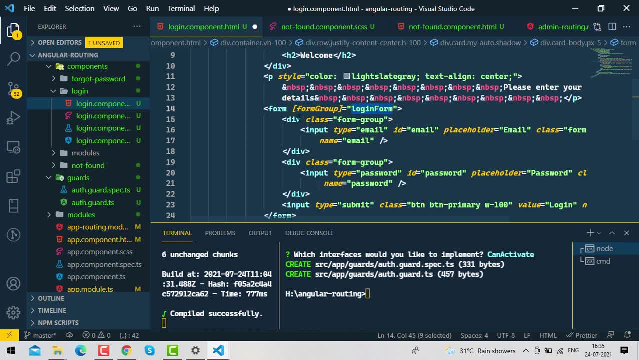 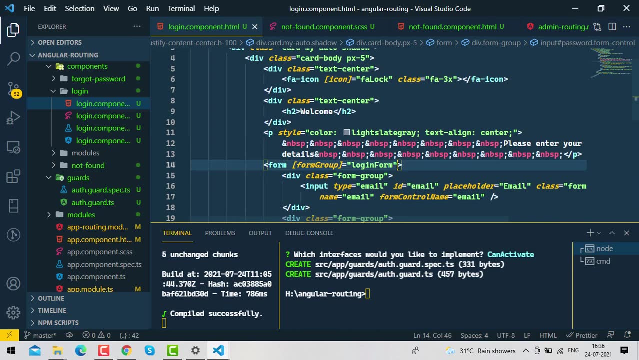 form group input. so here i'm passing login form object. so this is this object. so this is a form group object. so i'm passing here and now. we need to bind form control email in the same way for password. now one more thing inside the form attribute: so ng submit. so when user will click on submit button, this event will fire. so we. 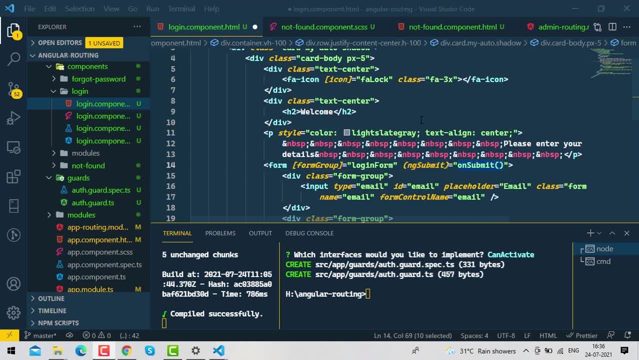 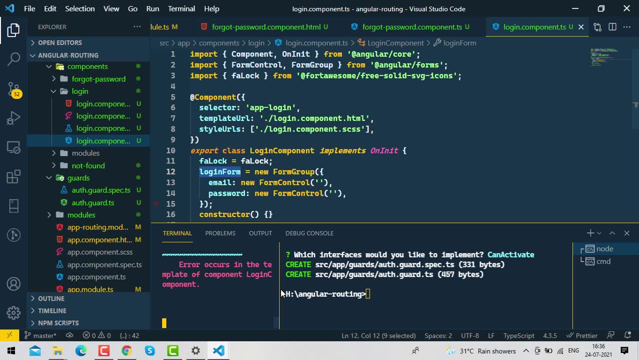 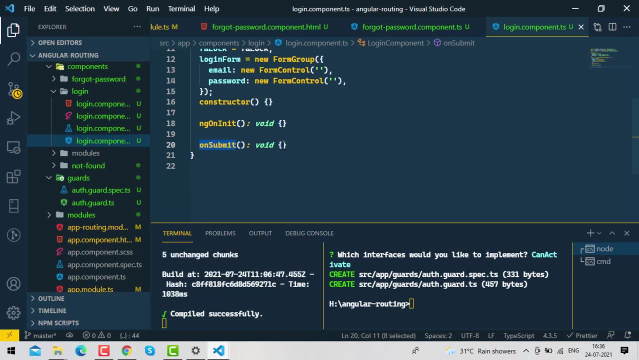 want to implement this on submit function, so let's create this function as well. so let's go to the login component. here you could see we are getting error because we haven't implemented on submit functions. okay, now, inside this, as of now, just write console dot log and see this dot form. 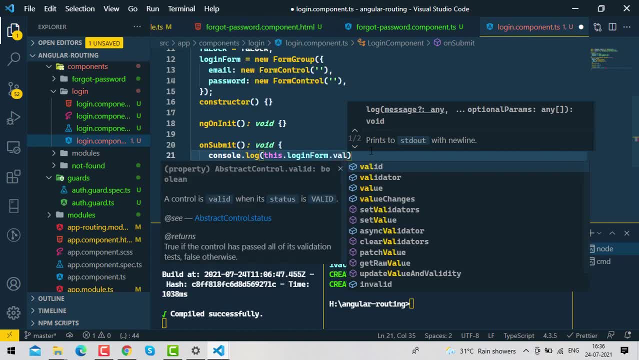 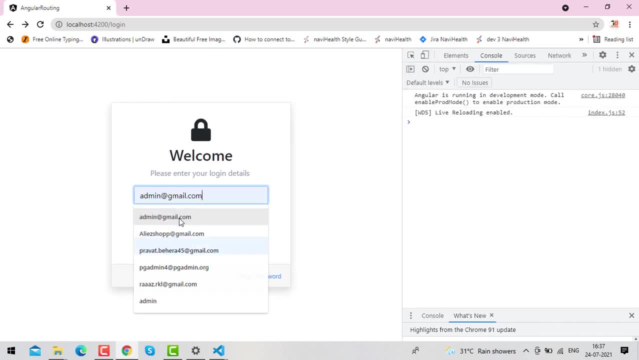 login from dot value. now let's go to and let me open console here and if we'll type admin and something here, if we'll click here, you could see we are getting this email and password. so we want to submit this email and password to the server for validations. so, finally, 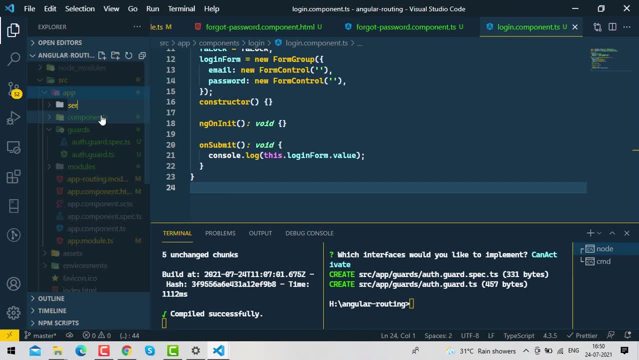 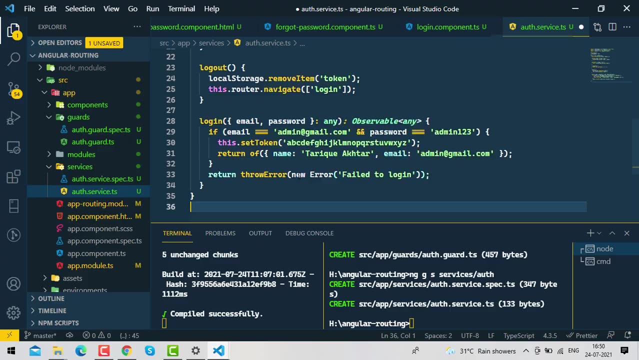 let's create a auth service. let me create one more folder services. let me generate ng generate service services. auth created auth service. so inside this you will find auth service. so let me implement all the logic here. so I have created all the auth related methods inside this service, like set token will. 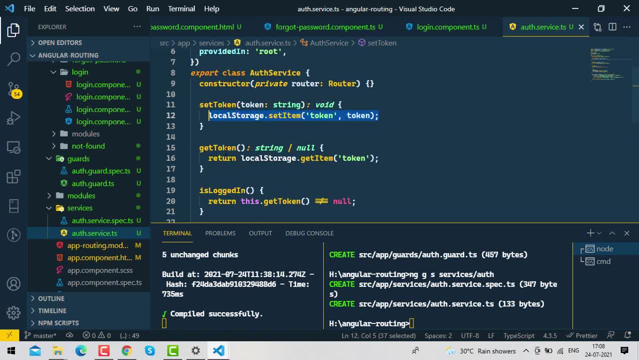 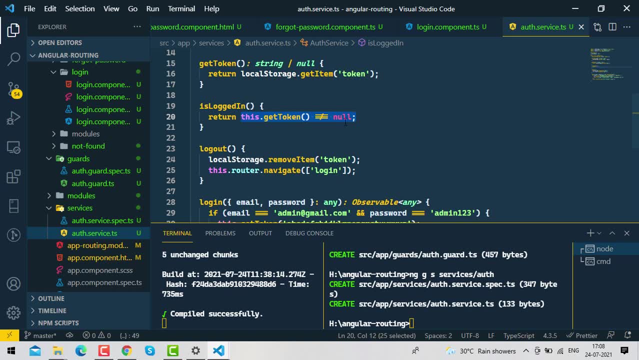 receive token and will store token inside a local storage. get token: will return token from local storage and is logged in. will check that token is present or not inside a local storage. but in a real-world situations you will check that token is valid or not. not. if token is valid, then you will return true. 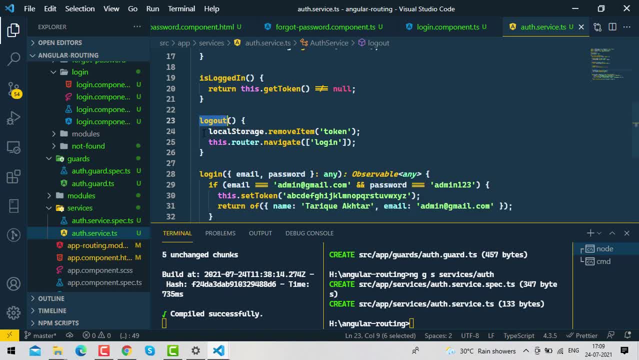 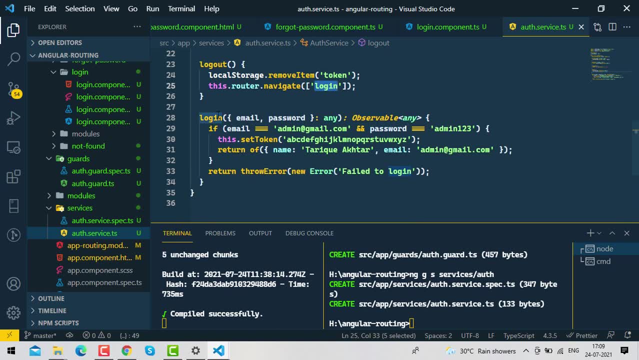 otherwise you will return false. in the same way I have implemented logout. here I'm just removing a token from local storage and navigating back user to login page. finally, login method. so here I'm just receiving one object that must have email and password and returning observable from this method. so here I'm. 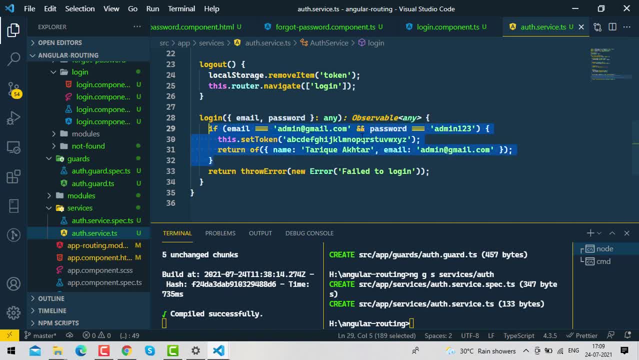 doing a static check, but in a real world you will connect this with API. so here I'm just checking that email is admin, at the rate gmailcom, and password admin. one, two, three. then we will store a token inside a local storage. a random token, password and email will not match. then we will read through an error from here. 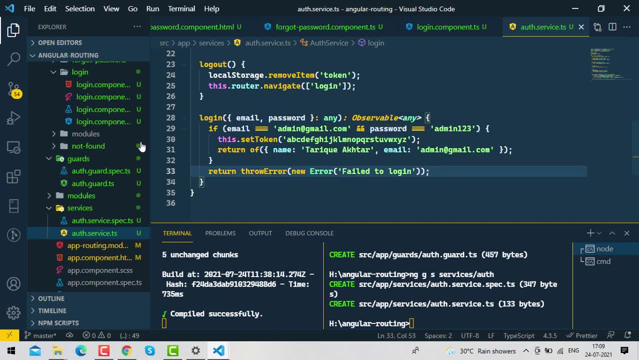 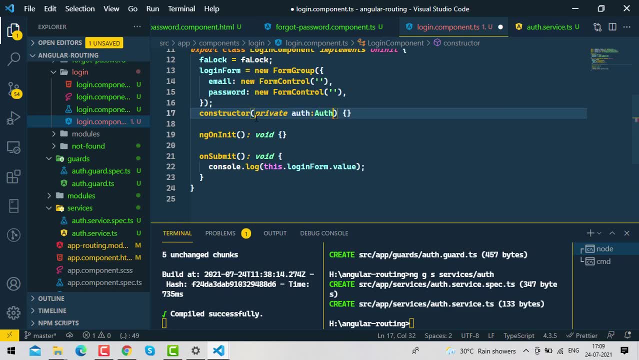 fail to login. now let's implement this service inside a login component. so first of all we need to inject this service inside this component: auth service. now let's write the logic inside on submit method. so here I'm just checking that form is valid or not. if form is valid, then we will submit this form value. 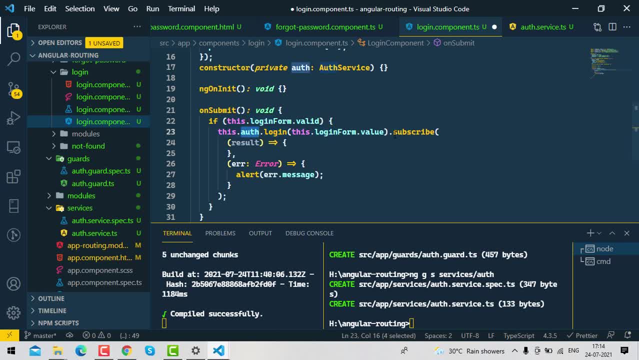 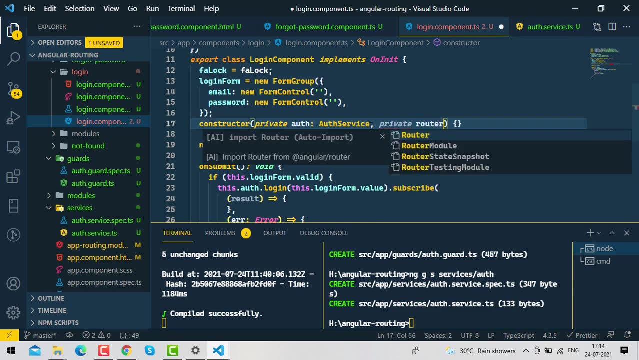 inside this login method of auth service and here I'm doing the subscribe. so if that is successful, then we will receive a result here and that if that is error, we will see an alert message. now one more thing we need: here private, let's me inject router and here let me write: 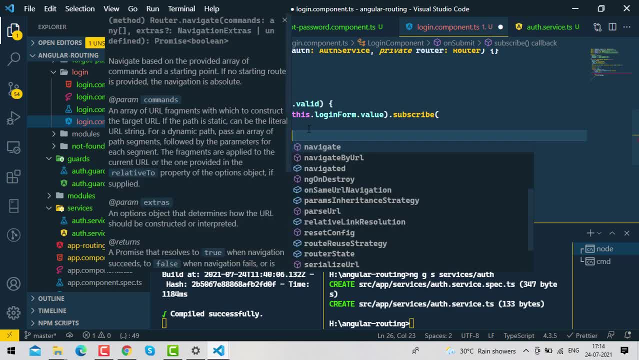 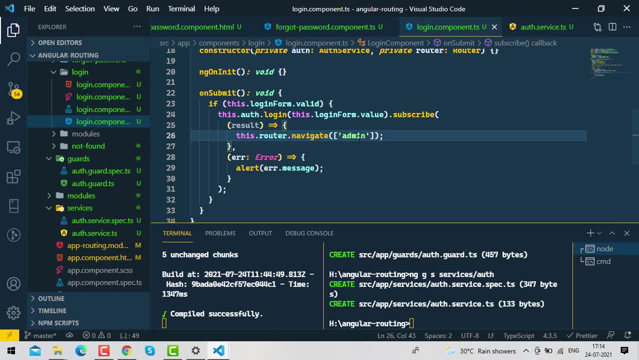 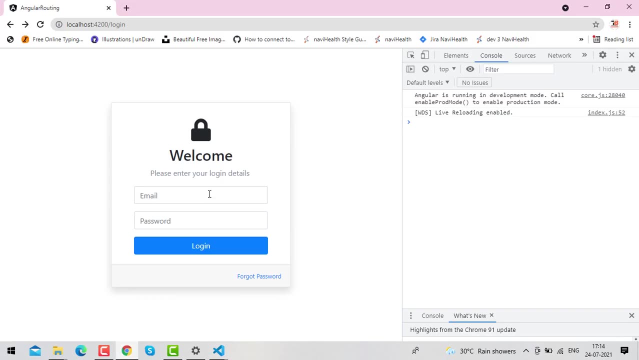 this: dot router dot. navigate admin. so if email and I email and password match, then we will navigate back user to admin dashboard. now let's check here. so it will pass admin and wrong password. then we can see that we get an alert message and fail to login. I will pass a correct. 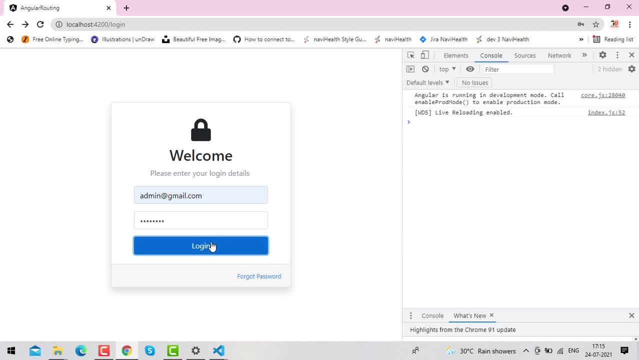 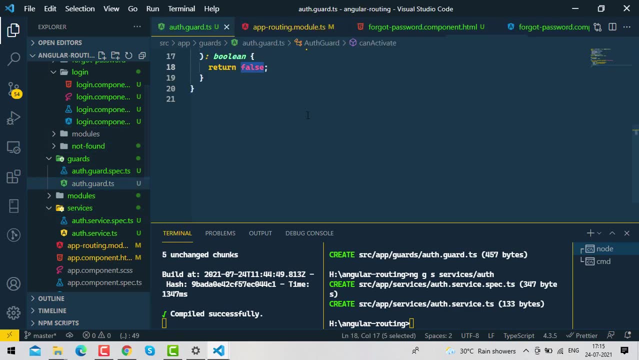 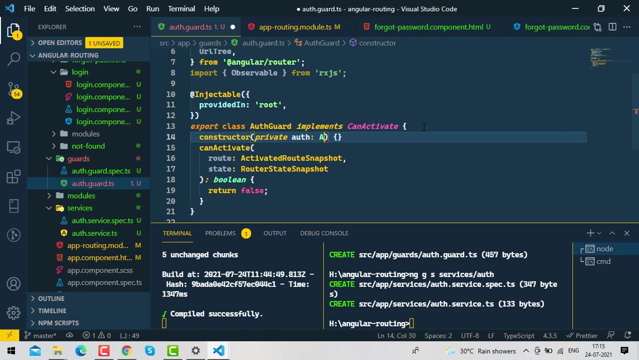 admin. one, two, three, then okay. so why we are not going to admin page? because we haven't implemented anything on guards. we are just returning false from here, so let's implement here as well. so we want to inject one service here, so we need to use constructor private auth service from. 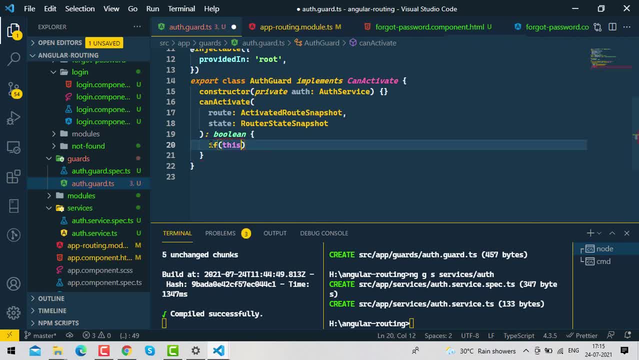 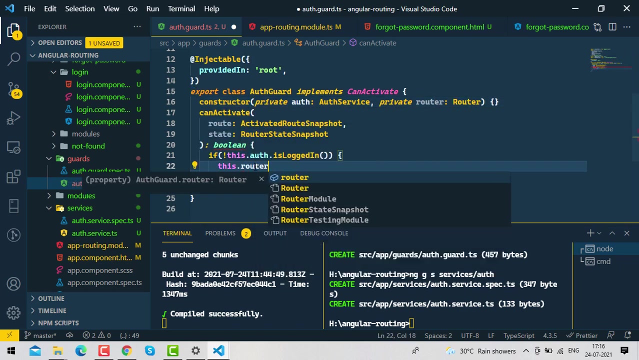 here. we just need to check that if this dot auth and we have is logged in. so if it returns false, then let's write a logic here. so this dot we want to navigate, so we need to implement one more thing here: private router, so we'll use routernavigate login. we are returning a true or false, so we need to return. 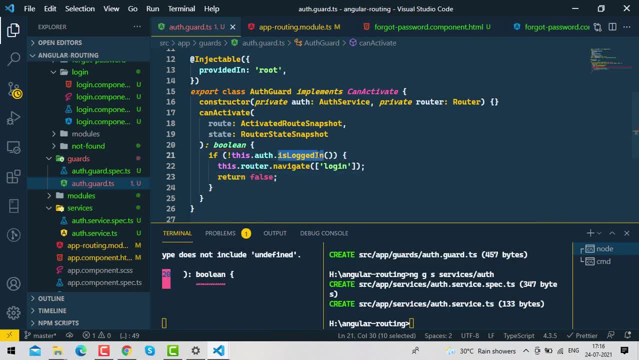 first here: false so is logged in. if returning false- so i'm just checking negation of that, so it will be true. so if user is not logged in, then we will redirect user to login page and we'll return false from here. return this dot: auth dot is logged in function. that's all, just let's. 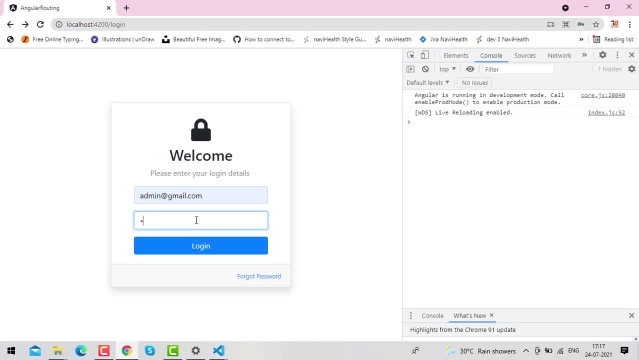 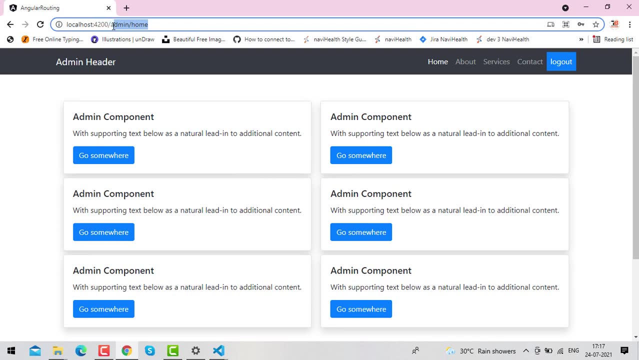 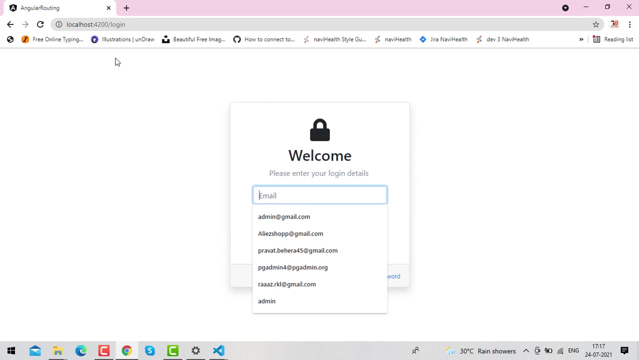 check right now. if admin now here, you could see we are able to go to the dashboard now. if we'll try to go to the login page again, we can. we can go back to the login, but we don't want user. once user is authenticated, we will block. 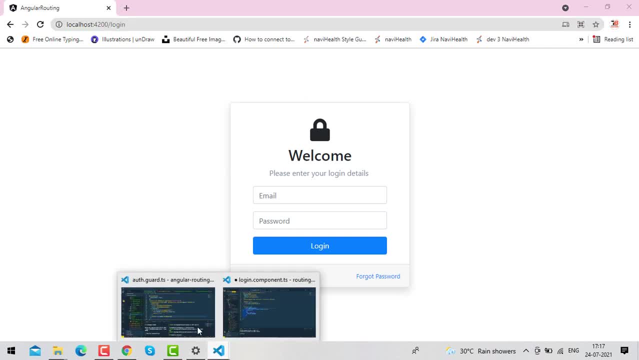 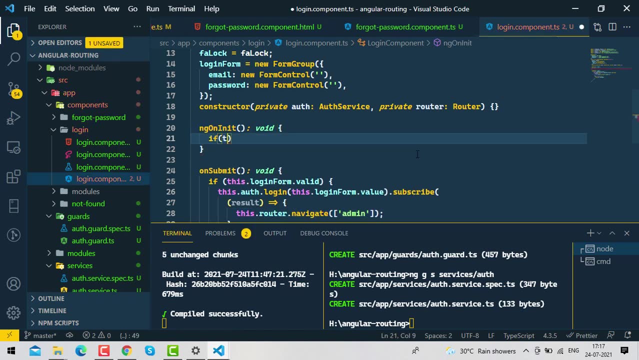 the users to come here inside the login page. so let's go to the login component and inside this ng on init, let's implement that. we will first check if this dot auth dot is logged in. if user is already logged in, then this dot router dot navigate user back to admin. 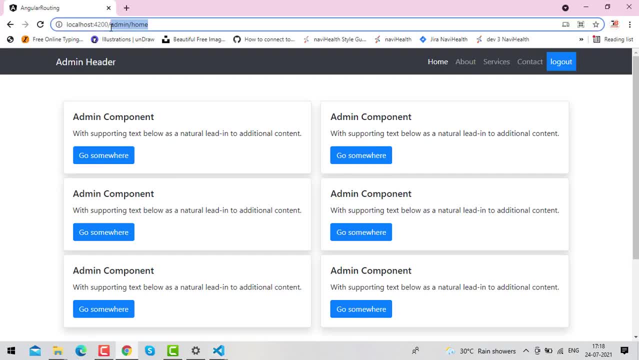 now. let's see now. user is already logged in. now. if i will try to go to login page now, here you could see it's redirecting me back to the admin. now i can't go back to the login unless and until we will not delete the tokens from local storage. so we haven't implemented a logout functions.